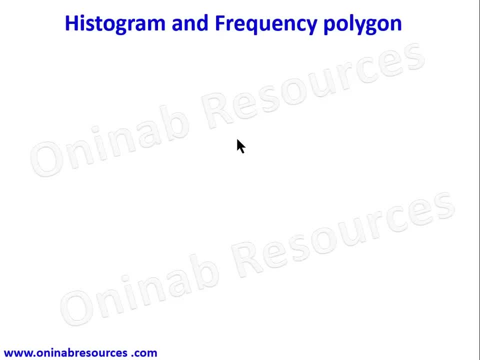 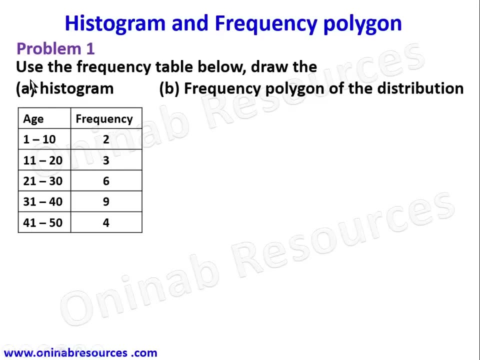 Hello out there. Welcome to this tutorial on histogram and frequency polygon. So we start the first problem, Problem 1. Use the frequency table below. Draw the histogram B- frequency polygon of the distribution. To draw a histogram we need the class boundaries of each of the class intervals. So here we are going to create additional column for class boundary. We call it CB. 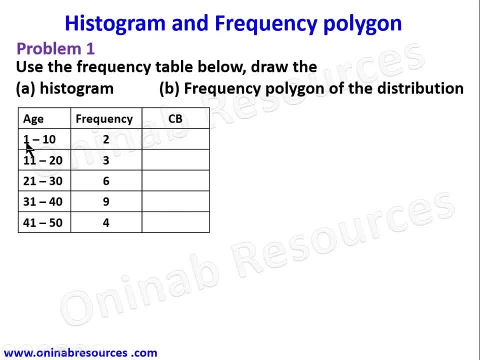 To get the class boundary here, we assume there is a number 0 before 1.. We are going to find the midpoint of 0 and 1.. To get the midpoint of 0 and 1, we are going to find the midpoint of 0 and 1.. 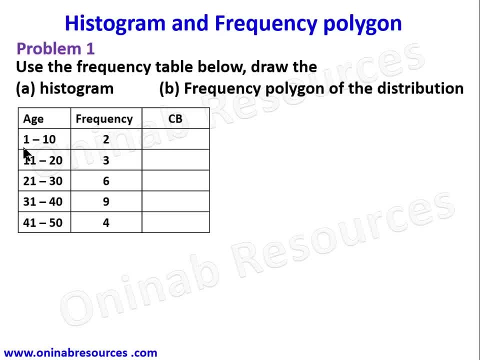 To get the midpoint of 0 and 1, we assume there is a number 0 before 1.. We are going to find the midpoint of 0 and 1.. To get the midpoint of 0 and 1, we assume there is a number 0 before 1.. We are going to find the midpoint of 0 and 1.. 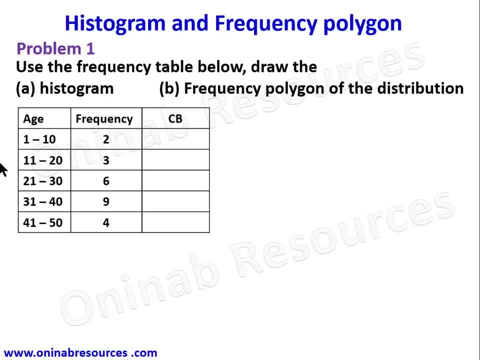 To get the midpoint of 0 and 1, we assume there is a number 0 before 1.. We are going to find the midpoint of 0 and 1.. To get the midpoint of 0 and 1, we assume there is a number 0 before 1.. We are going to find the midpoint of 0 and 1.. 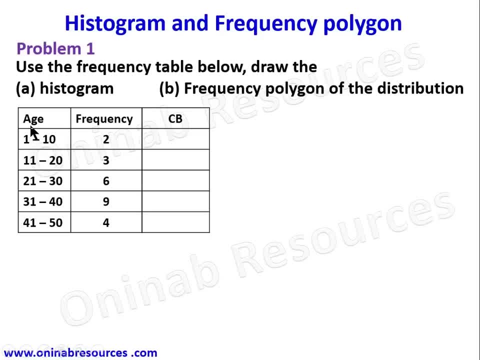 To get the midpoint of 0 and 1, we assume there is a number 0 before 1.. We are going to find the midpoint of 0 and 1.. To get the midpoint of 0 and 1, we assume there is a number 0 before 1.. We are going to find the midpoint of 0 and 1.. 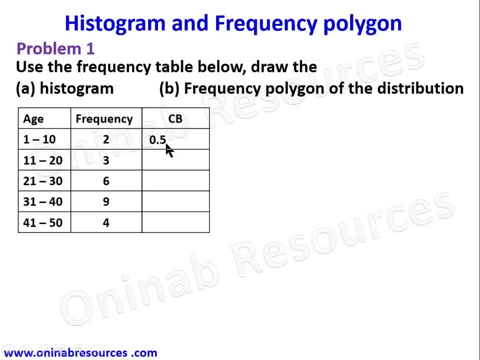 To get the midpoint of 0 and 1, we assume there is a number 0 before 1.. We are going to find the midpoint of 0 and 1.. To get the midpoint of 0 and 1, we assume there is a number 0 before 1.. We are going to find the midpoint of 0 and 1.. 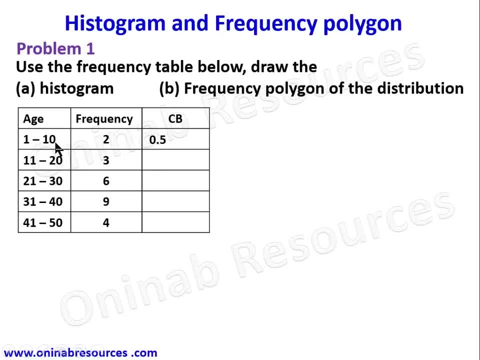 To get the midpoint of 0 and 1, we assume there is a number 0 before 1.. We are going to find the midpoint of 0 and 1.. To get the midpoint of 0 and 1, we assume there is a number 0 before 1.. We are going to find the midpoint of 0 and 1.. 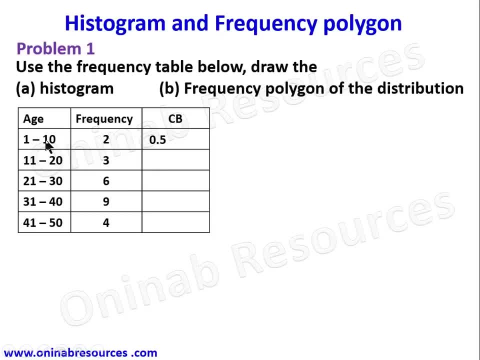 To get the midpoint of 0 and 1, we assume there is a number 0 before 1.. We are going to find the midpoint of 0 and 1.. To get the midpoint of 0 and 1, we assume there is a number 0 before 1.. We are going to find the midpoint of 0 and 1.. 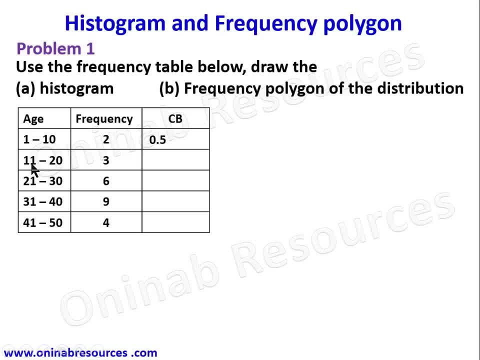 To get the midpoint of 0 and 1, we assume there is a number 0 before 1.. We are going to find the midpoint of 0 and 1.. To get the midpoint of 0 and 1, we assume there is a number 0 before 1.. We are going to find the midpoint of 0 and 1.. 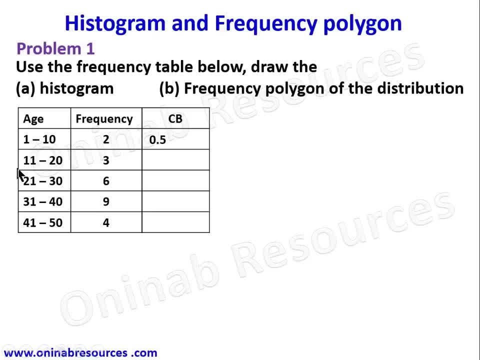 To get the midpoint of 0 and 1, we assume there is a number 0 before 1.. We are going to find the midpoint of 0 and 1.. To get the midpoint of 0 and 1, we assume there is a number 0 before 1.. We are going to find the midpoint of 0 and 1.. 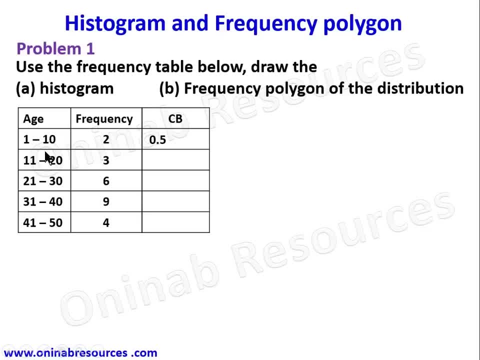 To get the midpoint of 0 and 1, we assume there is a number 0 before 1.. We are going to find the midpoint of 0 and 1.. To get the midpoint of 0 and 1, we assume there is a number 0 before 1.. We are going to find the midpoint of 0 and 1.. 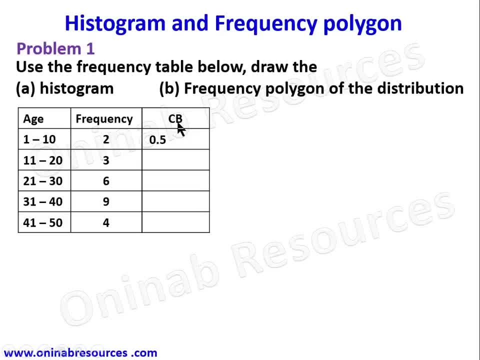 To get the midpoint of 0 and 1, we assume there is a number 0 before 1.. We are going to find the midpoint of 0 and 1.. To get the midpoint of 0 and 1, we assume there is a number 0 before 1.. We are going to find the midpoint of 0 and 1.. 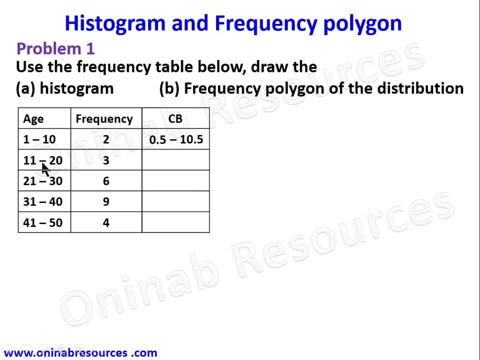 To get the midpoint of 0 and 1, we assume there is a number 0 before 1.. We are going to find the midpoint of 0 and 1.. To get the midpoint of 0 and 1, we assume there is a number 0 before 1.. We are going to find the midpoint of 0 and 1.. 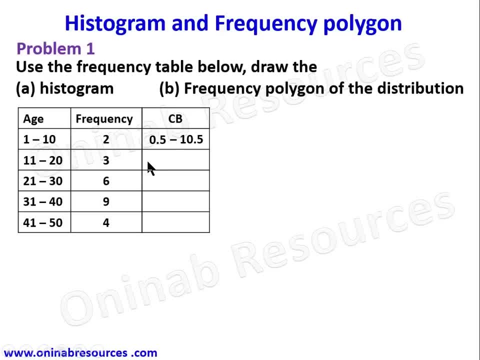 To get the midpoint of 0 and 1, we assume there is a number 0 before 1.. We are going to find the midpoint of 0 and 1.. To get the midpoint of 0 and 1, we assume there is a number 0 before 1.. We are going to find the midpoint of 0 and 1.. 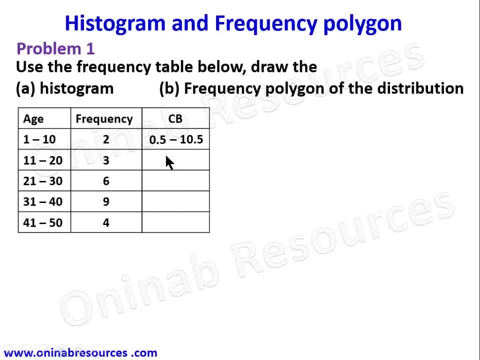 To get the midpoint of 0 and 1, we assume there is a number 0 before 1.. We are going to find the midpoint of 0 and 1.. To get the midpoint of 0 and 1, we assume there is a number 0 before 1.. We are going to find the midpoint of 0 and 1.. 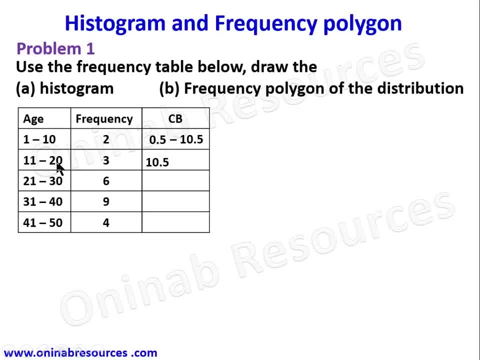 To get the midpoint of 0 and 1, we assume there is a number 0 before 1.. We are going to find the midpoint of 0 and 1.. To get the midpoint of 0 and 1, we assume there is a number 0 before 1.. We are going to find the midpoint of 0 and 1.. 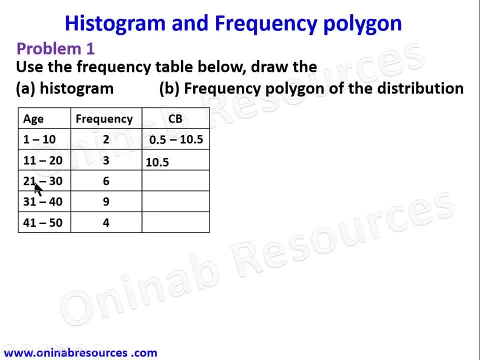 To get the midpoint of 0 and 1, we assume there is a number 0 before 1.. We are going to find the midpoint of 0 and 1.. To get the midpoint of 0 and 1, we assume there is a number 0 before 1.. We are going to find the midpoint of 0 and 1.. 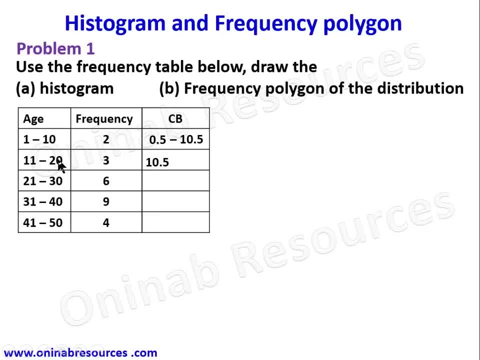 To get the midpoint of 0 and 1, we assume there is a number 0 before 1.. We are going to find the midpoint of 0 and 1.. To get the midpoint of 0 and 1, we assume there is a number 0 before 1.. We are going to find the midpoint of 0 and 1.. 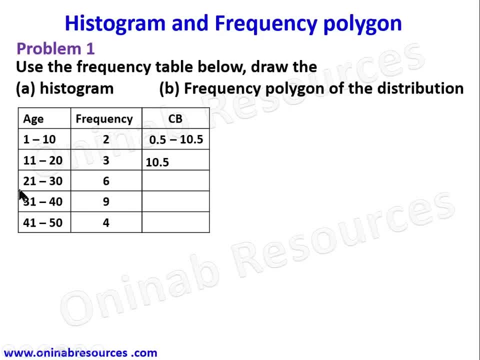 To get the midpoint of 0 and 1, we assume there is a number 0 before 1.. We are going to find the midpoint of 0 and 1.. To get the midpoint of 0 and 1, we assume there is a number 0 before 1.. We are going to find the midpoint of 0 and 1.. 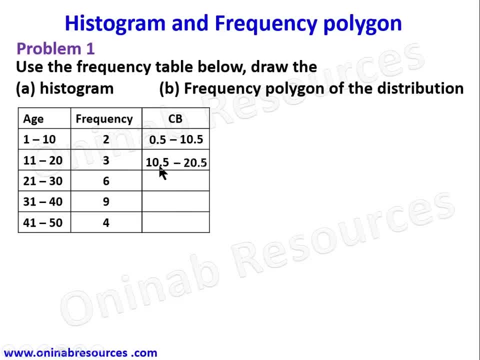 To get the midpoint of 0 and 1, we assume there is a number 0 before 1.. We are going to find the midpoint of 0 and 1.. To get the midpoint of 0 and 1, we assume there is a number 0 before 1.. We are going to find the midpoint of 0 and 1.. 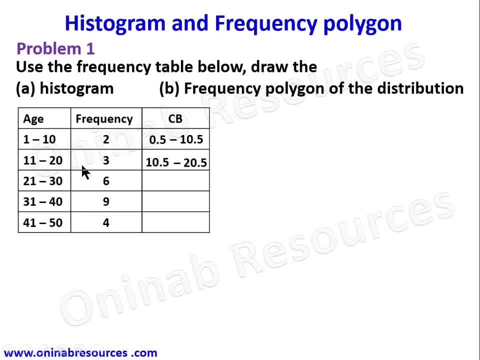 To get the midpoint of 0 and 1, we assume there is a number 0 before 1.. We are going to find the midpoint of 0 and 1.. To get the midpoint of 0 and 1, we assume there is a number 0 before 1.. We are going to find the midpoint of 0 and 1.. 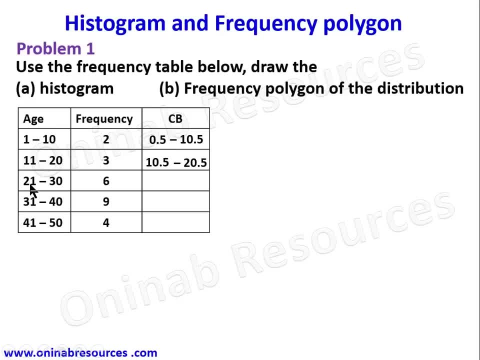 To get the midpoint of 0 and 1, we assume there is a number 0 before 1.. We are going to find the midpoint of 0 and 1.. To get the midpoint of 0 and 1, we assume there is a number 0 before 1.. We are going to find the midpoint of 0 and 1.. 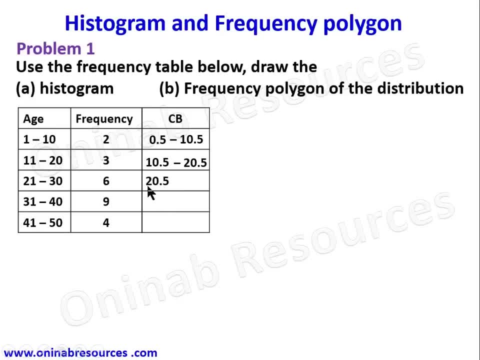 To get the midpoint of 0 and 1, we assume there is a number 0 before 1.. We are going to find the midpoint of 0 and 1.. To get the midpoint of 0 and 1, we assume there is a number 0 before 1.. We are going to find the midpoint of 0 and 1.. 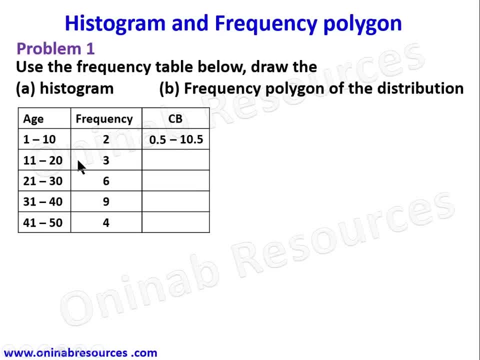 boundary here will be 10.5. so this 10.5 will automatically be the lower class boundary of the class immediately after it, which is going to give us 10.5. to get the upper class boundary of that class, 20 plus 21 gives 41. divided by 2 gives 21.5. that is the midpoint of 20 and 21. 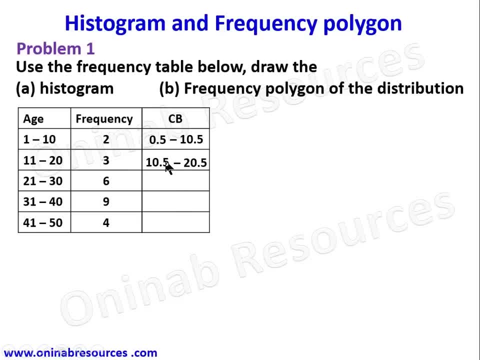 which forms the upper class boundary of the class interval 11 to 20.. this upper class boundary here becomes automatically the lower class boundary of the class immediately after each. and to get the upper class boundary for that class interval we said 30 plus 31 divided by 2, which gives 30.5. so so the class boundary there. 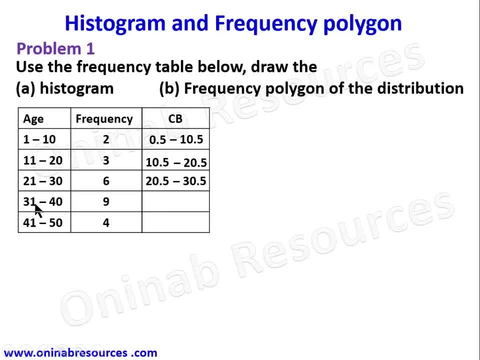 is 20.5 to 30.5 and the next class interval, the 30.5, automatically becomes the lower class boundary of the next class interval. and to get the upper class interval for that class, 40 plus 41 gives 81. 81 divided by 2 gives 40.5. that automatically becomes the lower class boundary. 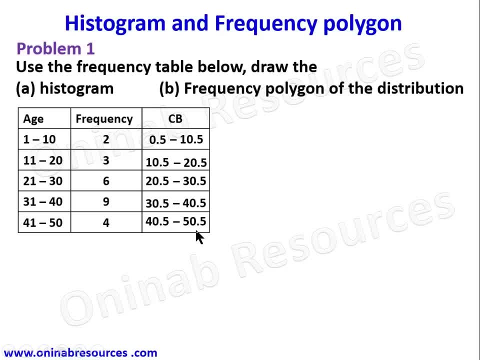 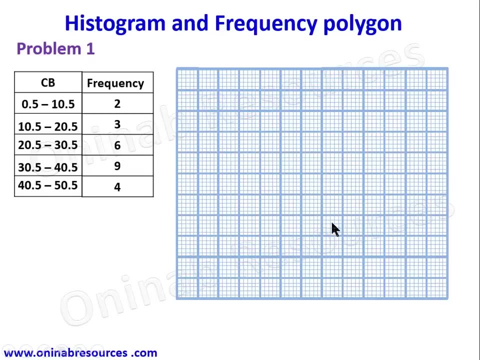 here to 50.5. so we are going to be using this frequency and the class boundary to draw the histogram of this distribution. we get our graph here. so, getting our graph, we have this as the class boundary and here is the frequency for the class boundary. we are starting from 0.5. 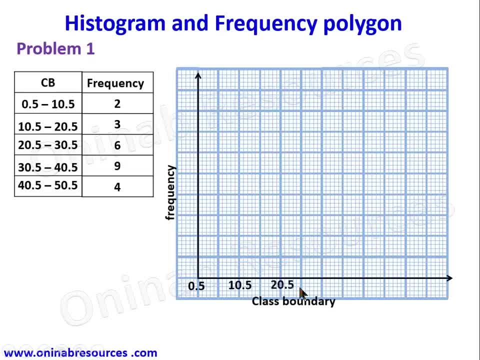 to 10.5, 10.5 to 20.5 to 30.5, 40.5 and 50.5 for the frequency. we start with zero here: one, two, three, four, five, six, seven, eight and nine. so we have the highest frequency of nine there. 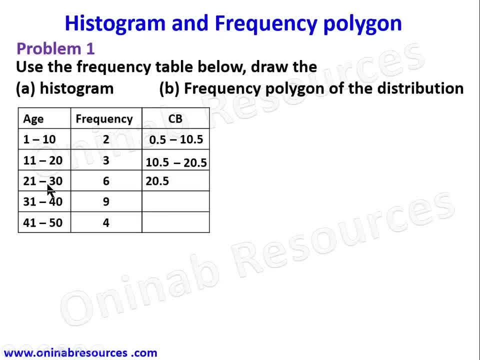 To get the midpoint of 0 and 1, we assume there is a number 0 before 1.. We are going to find the midpoint of 0 and 1.. To get the midpoint of 0 and 1, we assume there is a number 0 before 1.. We are going to find the midpoint of 0 and 1.. 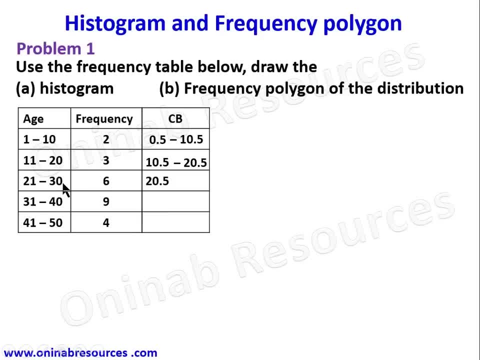 To get the midpoint of 0 and 1, we assume there is a number 0 before 1.. We are going to find the midpoint of 0 and 1.. To get the midpoint of 0 and 1, we assume there is a number 0 before 1.. We are going to find the midpoint of 0 and 1.. 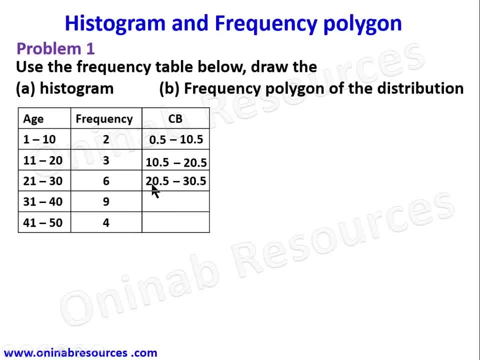 To get the midpoint of 0 and 1, we assume there is a number 0 before 1.. We are going to find the midpoint of 0 and 1.. To get the midpoint of 0 and 1, we assume there is a number 0 before 1.. We are going to find the midpoint of 0 and 1.. 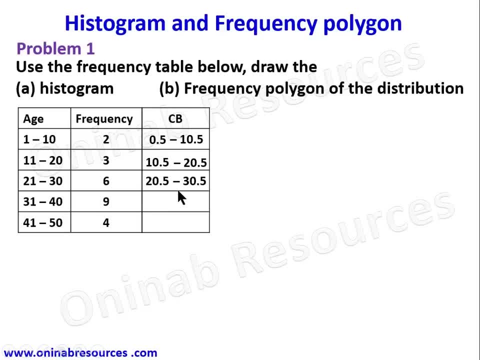 To get the midpoint of 0 and 1, we assume there is a number 0 before 1.. We are going to find the midpoint of 0 and 1.. To get the midpoint of 0 and 1, we assume there is a number 0 before 1.. We are going to find the midpoint of 0 and 1.. 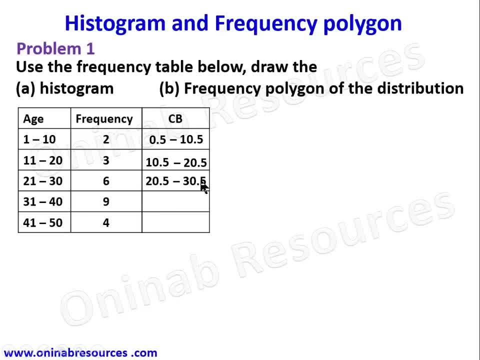 To get the midpoint of 0 and 1, we assume there is a number 0 before 1.. We are going to find the midpoint of 0 and 1.. To get the midpoint of 0 and 1, we assume there is a number 0 before 1.. We are going to find the midpoint of 0 and 1.. 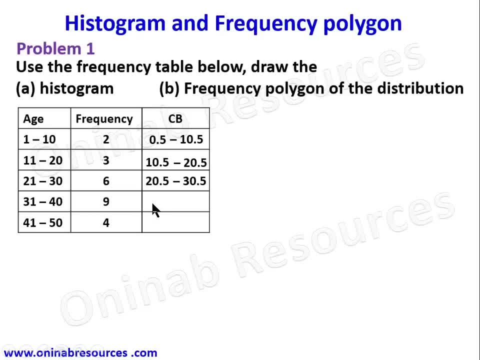 To get the midpoint of 0 and 1, we assume there is a number 0 before 1.. We are going to find the midpoint of 0 and 1.. To get the midpoint of 0 and 1, we assume there is a number 0 before 1.. We are going to find the midpoint of 0 and 1.. 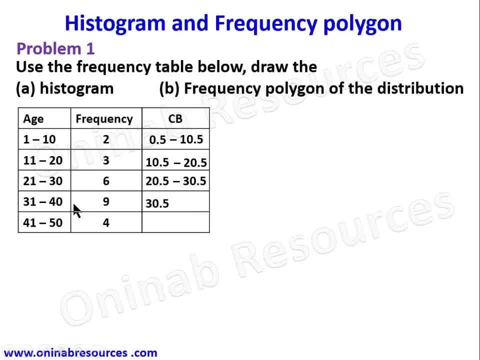 To get the midpoint of 0 and 1, we assume there is a number 0 before 1.. We are going to find the midpoint of 0 and 1.. To get the midpoint of 0 and 1, we assume there is a number 0 before 1.. We are going to find the midpoint of 0 and 1.. 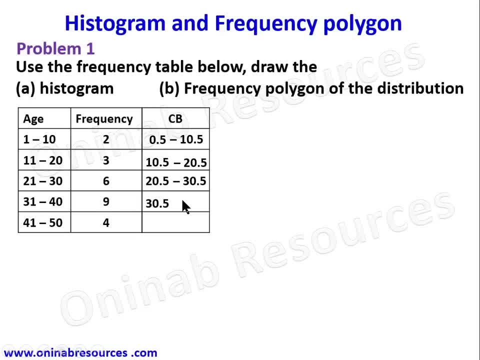 To get the midpoint of 0 and 1, we assume there is a number 0 before 1.. We are going to find the midpoint of 0 and 1.. To get the midpoint of 0 and 1, we assume there is a number 0 before 1.. We are going to find the midpoint of 0 and 1.. 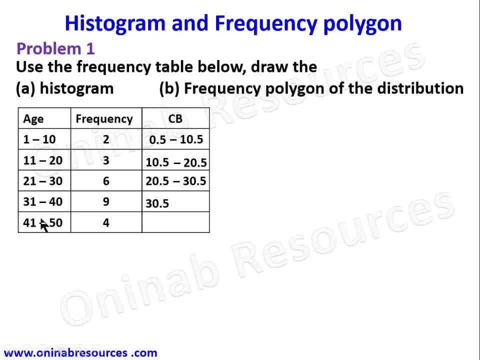 To get the midpoint of 0 and 1, we assume there is a number 0 before 1.. We are going to find the midpoint of 0 and 1.. To get the midpoint of 0 and 1, we assume there is a number 0 before 1.. We are going to find the midpoint of 0 and 1.. 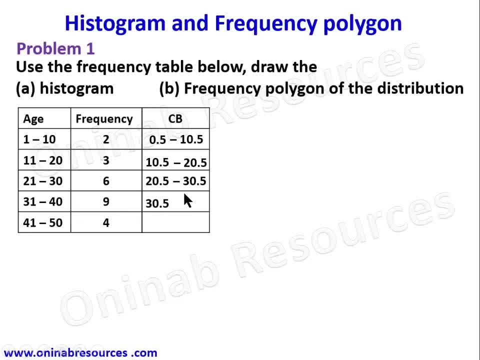 To get the midpoint of 0 and 1, we assume there is a number 0 before 1.. We are going to find the midpoint of 0 and 1.. To get the midpoint of 0 and 1, we assume there is a number 0 before 1.. We are going to find the midpoint of 0 and 1.. 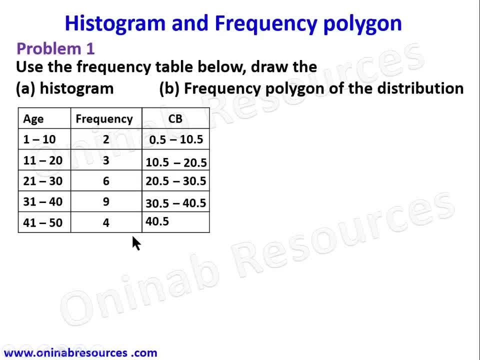 To get the midpoint of 0 and 1, we assume there is a number 0 before 1.. We are going to find the midpoint of 0 and 1.. To get the midpoint of 0 and 1, we assume there is a number 0 before 1.. We are going to find the midpoint of 0 and 1.. 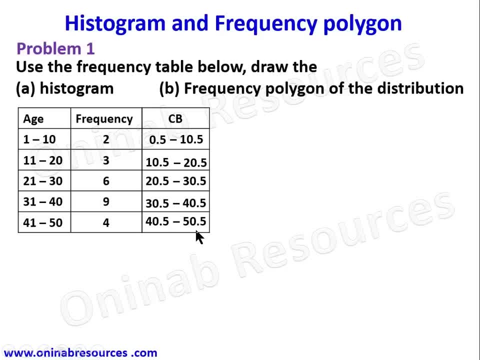 To get the midpoint of 0 and 1, we assume there is a number 0 before 1.. We are going to find the midpoint of 0 and 1.. To get the midpoint of 0 and 1, we assume there is a number 0 before 1.. We are going to find the midpoint of 0 and 1.. 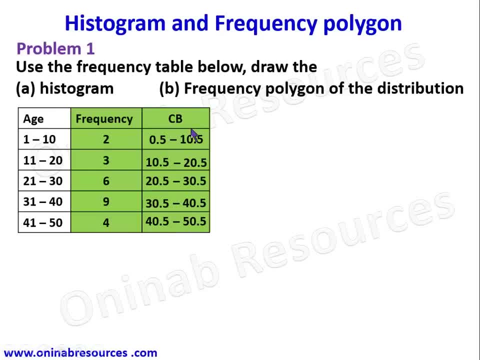 To get the midpoint of 0 and 1, we assume there is a number 0 before 1.. We are going to find the midpoint of 0 and 1.. To get the midpoint of 0 and 1, we assume there is a number 0 before 1.. We are going to find the midpoint of 0 and 1.. 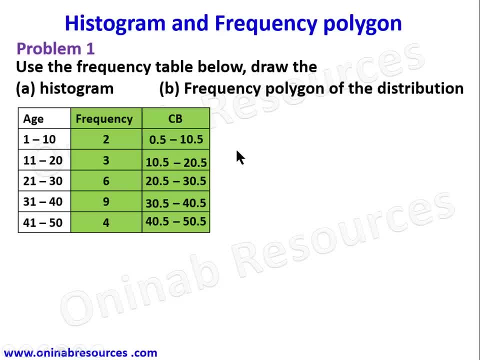 To get the midpoint of 0 and 1, we assume there is a number 0 before 1.. We are going to find the midpoint of 0 and 1.. To get the midpoint of 0 and 1, we assume there is a number 0 before 1.. We are going to find the midpoint of 0 and 1.. 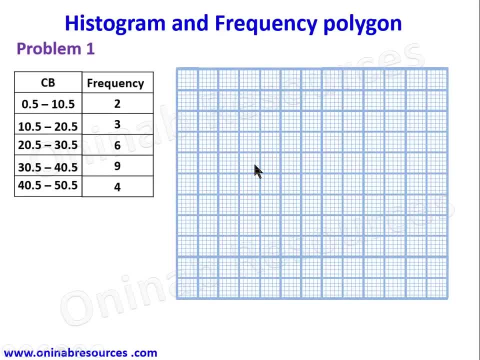 To get the midpoint of 0 and 1, we assume there is a number 0 before 1.. We are going to find the midpoint of 0 and 1.. To get the midpoint of 0 and 1, we assume there is a number 0 before 1.. We are going to find the midpoint of 0 and 1.. 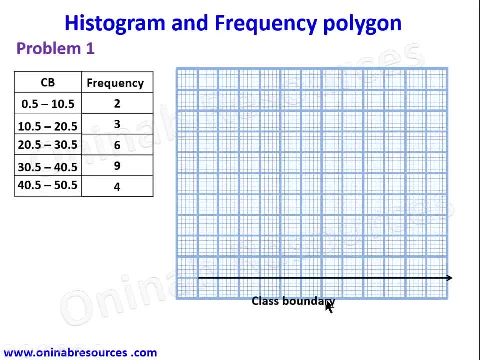 To get the midpoint of 0 and 1, we assume there is a number 0 before 1.. We are going to find the midpoint of 0 and 1.. To get the midpoint of 0 and 1, we assume there is a number 0 before 1.. We are going to find the midpoint of 0 and 1.. 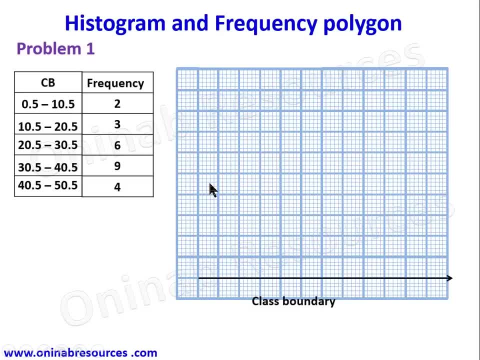 To get the midpoint of 0 and 1, we assume there is a number 0 before 1.. We are going to find the midpoint of 0 and 1.. To get the midpoint of 0 and 1, we assume there is a number 0 before 1.. We are going to find the midpoint of 0 and 1.. 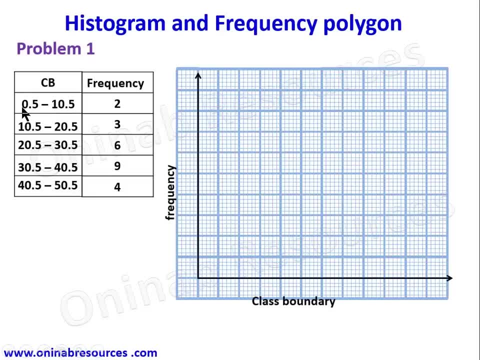 To get the midpoint of 0 and 1, we assume there is a number 0 before 1.. We are going to find the midpoint of 0 and 1.. To get the midpoint of 0 and 1, we assume there is a number 0 before 1.. We are going to find the midpoint of 0 and 1.. 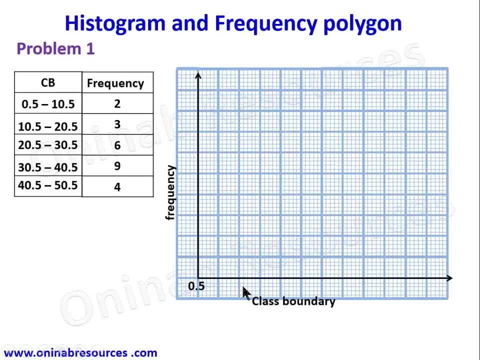 To get the midpoint of 0 and 1, we assume there is a number 0 before 1.. We are going to find the midpoint of 0 and 1.. To get the midpoint of 0 and 1, we assume there is a number 0 before 1.. We are going to find the midpoint of 0 and 1.. 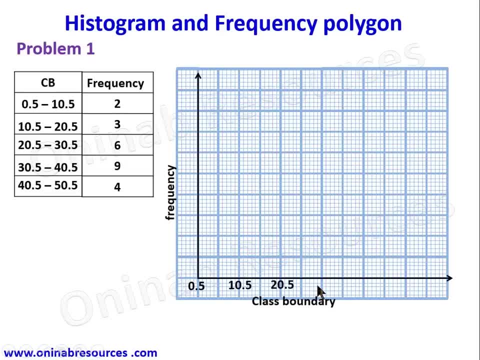 To get the midpoint of 0 and 1, we assume there is a number 0 before 1.. We are going to find the midpoint of 0 and 1.. To get the midpoint of 0 and 1, we assume there is a number 0 before 1.. We are going to find the midpoint of 0 and 1.. 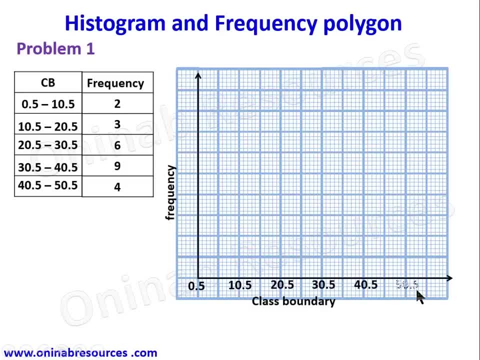 To get the midpoint of 0 and 1, we assume there is a number 0 before 1.. We are going to find the midpoint of 0 and 1.. To get the midpoint of 0 and 1, we assume there is a number 0 before 1.. We are going to find the midpoint of 0 and 1.. 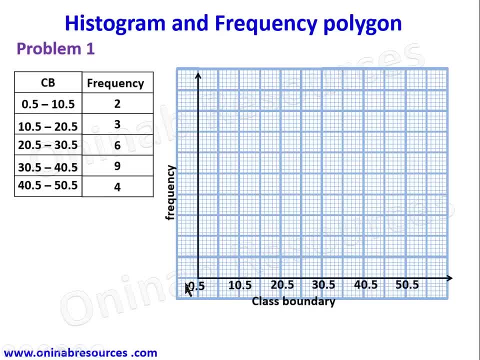 To get the midpoint of 0 and 1, we assume there is a number 0 before 1.. We are going to find the midpoint of 0 and 1.. To get the midpoint of 0 and 1, we assume there is a number 0 before 1.. We are going to find the midpoint of 0 and 1.. 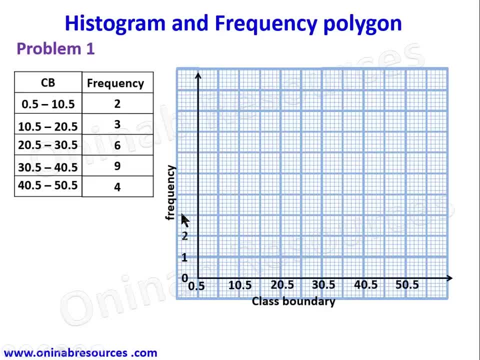 To get the midpoint of 0 and 1, we assume there is a number 0 before 1.. We are going to find the midpoint of 0 and 1.. To get the midpoint of 0 and 1, we assume there is a number 0 before 1.. We are going to find the midpoint of 0 and 1.. 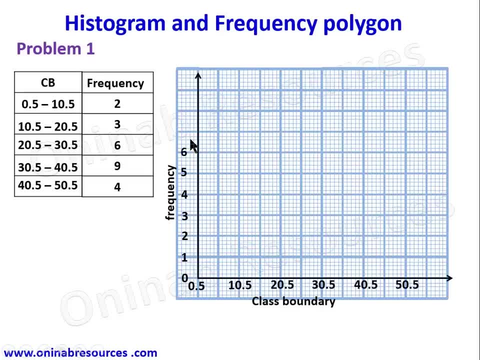 To get the midpoint of 0 and 1, we assume there is a number 0 before 1.. We are going to find the midpoint of 0 and 1.. To get the midpoint of 0 and 1, we assume there is a number 0 before 1.. We are going to find the midpoint of 0 and 1.. 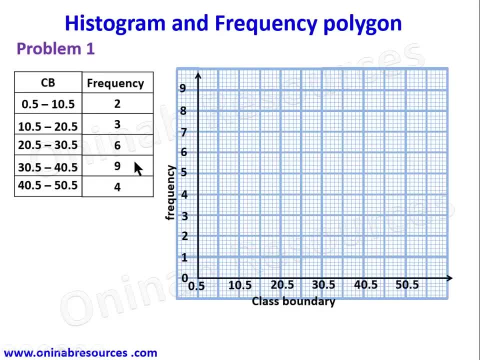 To get the midpoint of 0 and 1, we assume there is a number 0 before 1.. We are going to find the midpoint of 0 and 1.. To get the midpoint of 0 and 1, we assume there is a number 0 before 1.. We are going to find the midpoint of 0 and 1.. 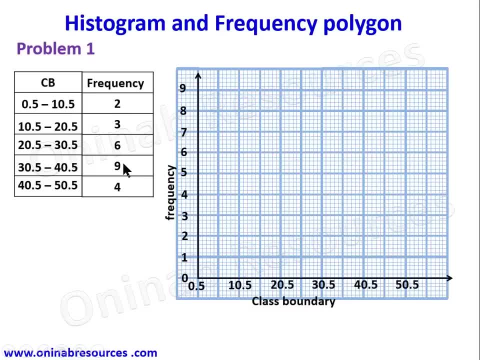 To get the midpoint of 0 and 1, we assume there is a number 0 before 1.. We are going to find the midpoint of 0 and 1.. To get the midpoint of 0 and 1, we assume there is a number 0 before 1.. We are going to find the midpoint of 0 and 1.. 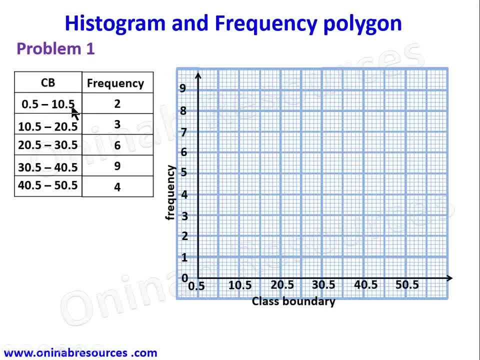 To get the midpoint of 0 and 1, we assume there is a number 0 before 1.. We are going to find the midpoint of 0 and 1.. To get the midpoint of 0 and 1, we assume there is a number 0 before 1.. We are going to find the midpoint of 0 and 1.. 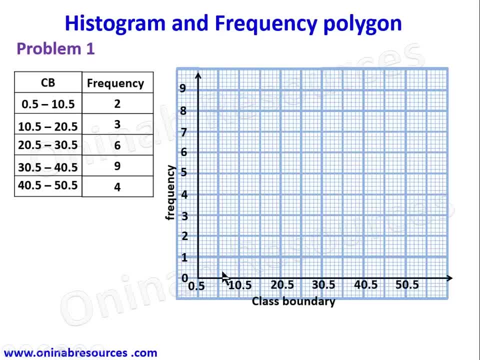 To get the midpoint of 0 and 1, we assume there is a number 0 before 1.. We are going to find the midpoint of 0 and 1.. To get the midpoint of 0 and 1, we assume there is a number 0 before 1.. We are going to find the midpoint of 0 and 1.. 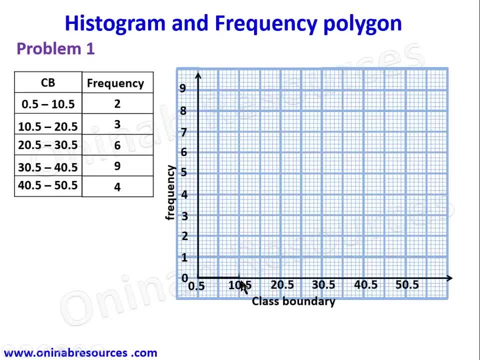 To get the midpoint of 0 and 1, we assume there is a number 0 before 1.. We are going to find the midpoint of 0 and 1.. To get the midpoint of 0 and 1, we assume there is a number 0 before 1.. We are going to find the midpoint of 0 and 1.. 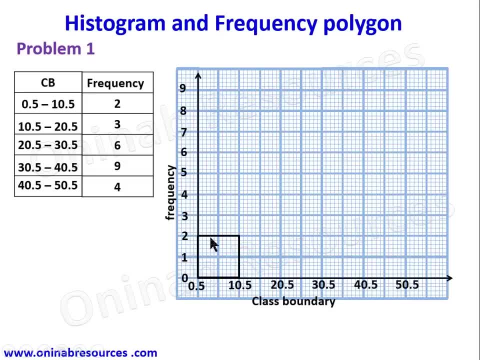 To get the midpoint of 0 and 1, we assume there is a number 0 before 1.. We are going to find the midpoint of 0 and 1.. To get the midpoint of 0 and 1, we assume there is a number 0 before 1.. We are going to find the midpoint of 0 and 1.. 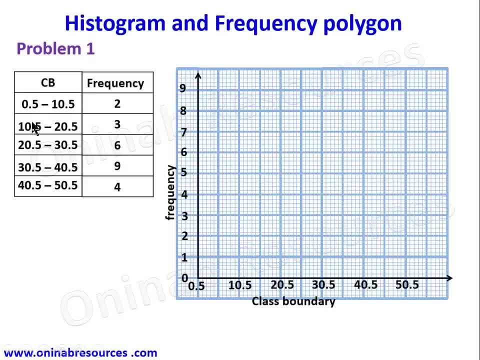 um, between 0.5 to 10.5 is two, the frequency is two. so from 0.5 to 10.5 we have the frequency to be two. so the height of the bar is the frequency, while the width is the class boundary, and again, from 10.5 to 20.5 it is. 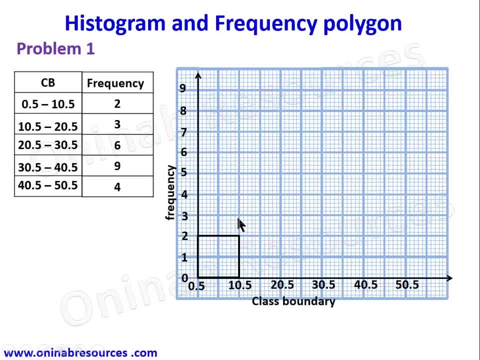 end to end bar. so we have it, the frequency to be 3. so it goes until we get to frequency 3, which gives the height of the bar, and for 20.5 to 30.5, again from 20.5 to 30.5, the frequency is 6. so the 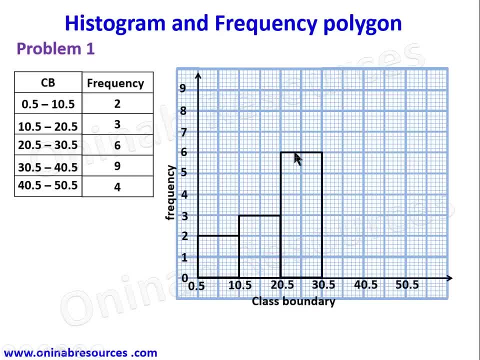 height of the bar will be 6, so we have that. then for 30.5 to 40.5, the frequency is 9, so the height of the bar will be 9. it stops here. and finally, for 40.5 to 50.5, so the height is 4. so we have it as 4 here. so we have succeeded in drawing the 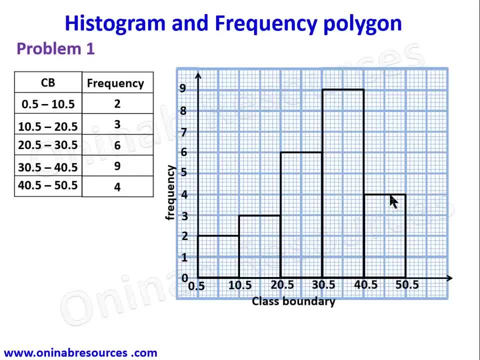 histogram of this distribution in our previous video on histogram. after drawing the histogram we estimated the mode from the histogram. to get the mode, we look at the tallest bar and from this angle we estimate the mode from the histogram. we estimate the mode from the histogram here where it touches the bar. before each we draw a line to the opposite. 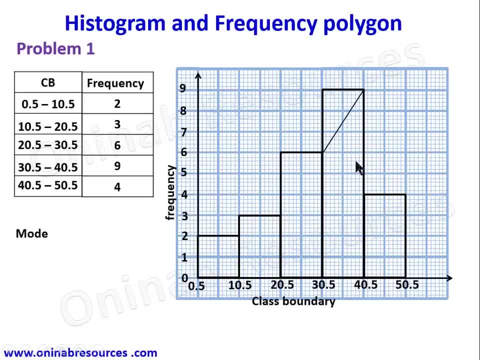 vertex. so we have it. and for where it touches the bar, after each we draw another line to join the opposite vertex. so we have it. then we now look at their points of intersection. the point of intersection is this: read it down to the class boundary axis: this is the point of intersection. and this is the point of intersection. 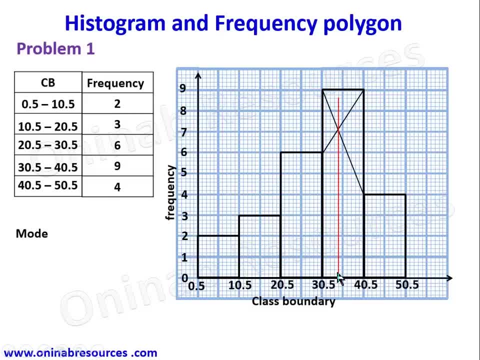 and this is the point of intersection, and this is the point of intersection. so you use both your will use one glued hard to join and this is both of your will you do, is you do, and have third, well, we have the second point: to join the horizontalStar and third one, 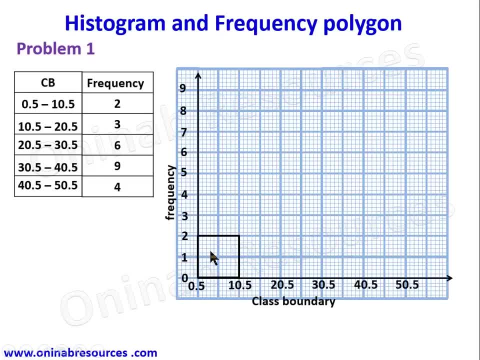 To get the midpoint of 0 and 1, we assume there is a number 0 before 1.. We are going to find the midpoint of 0 and 1.. To get the midpoint of 0 and 1, we assume there is a number 0 before 1.. We are going to find the midpoint of 0 and 1.. 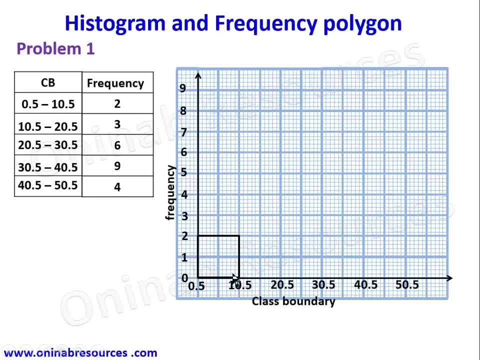 To get the midpoint of 0 and 1, we assume there is a number 0 before 1.. We are going to find the midpoint of 0 and 1.. To get the midpoint of 0 and 1, we assume there is a number 0 before 1.. We are going to find the midpoint of 0 and 1.. 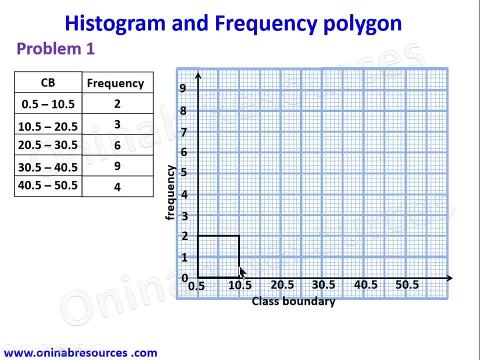 To get the midpoint of 0 and 1, we assume there is a number 0 before 1.. We are going to find the midpoint of 0 and 1.. To get the midpoint of 0 and 1, we assume there is a number 0 before 1.. We are going to find the midpoint of 0 and 1.. 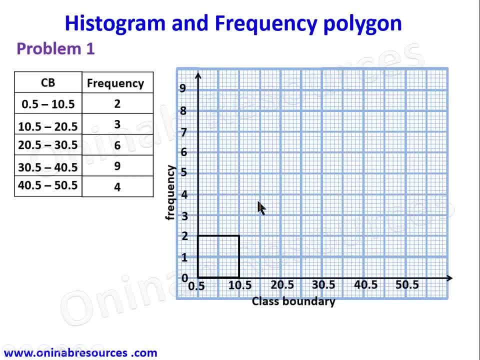 To get the midpoint of 0 and 1, we assume there is a number 0 before 1.. We are going to find the midpoint of 0 and 1.. To get the midpoint of 0 and 1, we assume there is a number 0 before 1.. We are going to find the midpoint of 0 and 1.. 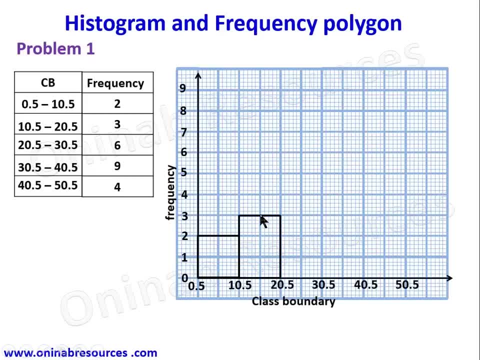 To get the midpoint of 0 and 1, we assume there is a number 0 before 1.. We are going to find the midpoint of 0 and 1.. To get the midpoint of 0 and 1, we assume there is a number 0 before 1.. We are going to find the midpoint of 0 and 1.. 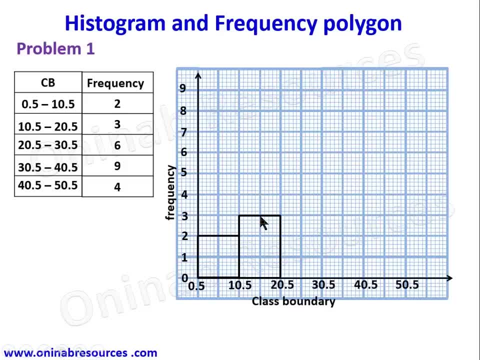 To get the midpoint of 0 and 1, we assume there is a number 0 before 1.. We are going to find the midpoint of 0 and 1.. To get the midpoint of 0 and 1, we assume there is a number 0 before 1.. We are going to find the midpoint of 0 and 1.. 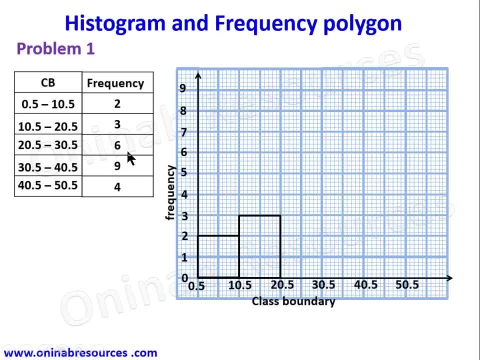 To get the midpoint of 0 and 1, we assume there is a number 0 before 1.. We are going to find the midpoint of 0 and 1.. To get the midpoint of 0 and 1, we assume there is a number 0 before 1.. We are going to find the midpoint of 0 and 1.. 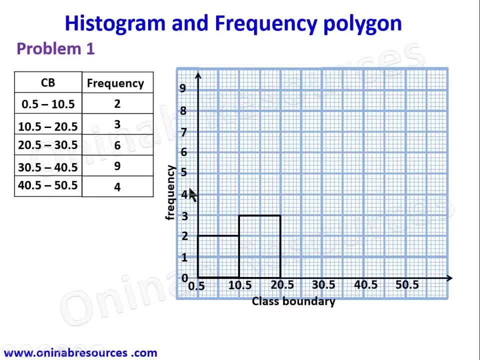 To get the midpoint of 0 and 1, we assume there is a number 0 before 1.. We are going to find the midpoint of 0 and 1.. To get the midpoint of 0 and 1, we assume there is a number 0 before 1.. We are going to find the midpoint of 0 and 1.. 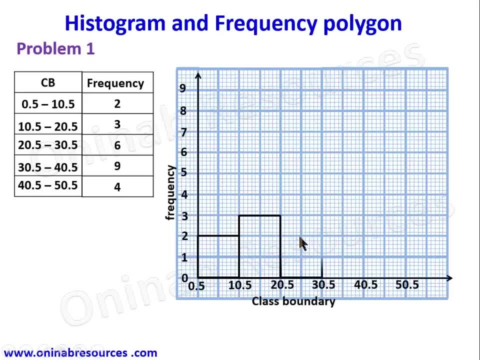 To get the midpoint of 0 and 1, we assume there is a number 0 before 1.. We are going to find the midpoint of 0 and 1.. To get the midpoint of 0 and 1, we assume there is a number 0 before 1.. We are going to find the midpoint of 0 and 1.. 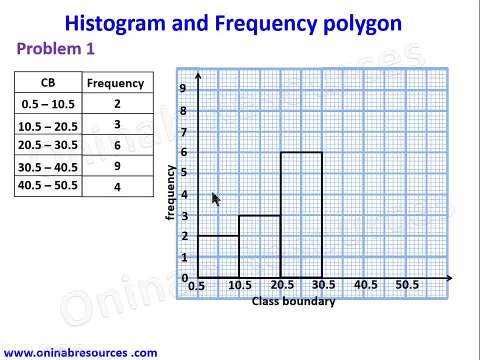 To get the midpoint of 0 and 1, we assume there is a number 0 before 1.. We are going to find the midpoint of 0 and 1.. To get the midpoint of 0 and 1, we assume there is a number 0 before 1.. We are going to find the midpoint of 0 and 1.. 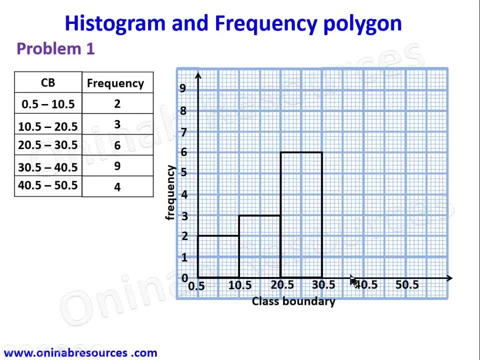 To get the midpoint of 0 and 1, we assume there is a number 0 before 1.. We are going to find the midpoint of 0 and 1.. To get the midpoint of 0 and 1, we assume there is a number 0 before 1.. We are going to find the midpoint of 0 and 1.. 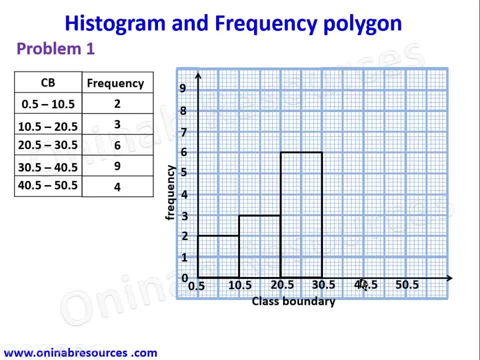 To get the midpoint of 0 and 1, we assume there is a number 0 before 1.. We are going to find the midpoint of 0 and 1.. To get the midpoint of 0 and 1, we assume there is a number 0 before 1.. We are going to find the midpoint of 0 and 1.. 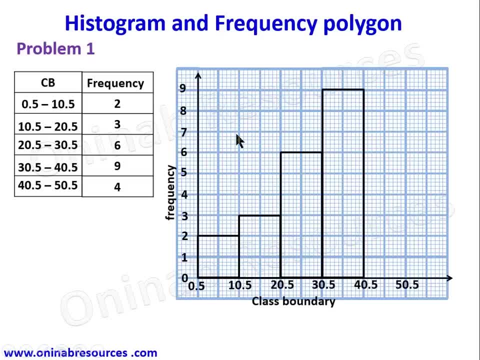 To get the midpoint of 0 and 1, we assume there is a number 0 before 1.. We are going to find the midpoint of 0 and 1.. To get the midpoint of 0 and 1, we assume there is a number 0 before 1.. We are going to find the midpoint of 0 and 1.. 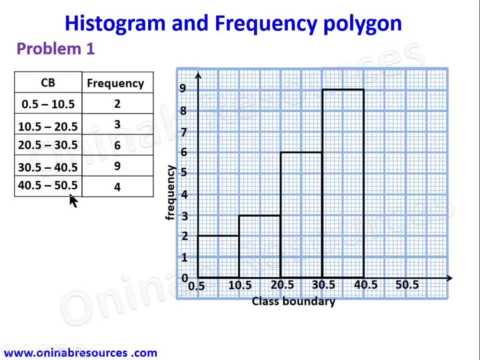 To get the midpoint of 0 and 1, we assume there is a number 0 before 1.. We are going to find the midpoint of 0 and 1.. To get the midpoint of 0 and 1, we assume there is a number 0 before 1.. We are going to find the midpoint of 0 and 1.. 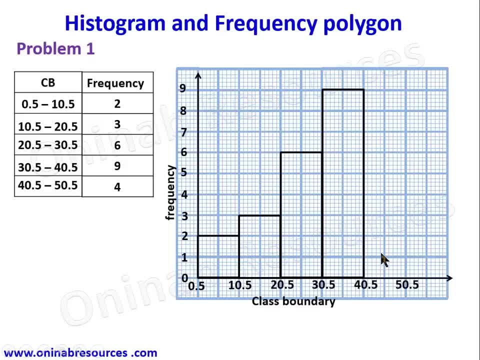 To get the midpoint of 0 and 1, we assume there is a number 0 before 1.. We are going to find the midpoint of 0 and 1.. To get the midpoint of 0 and 1, we assume there is a number 0 before 1.. We are going to find the midpoint of 0 and 1.. 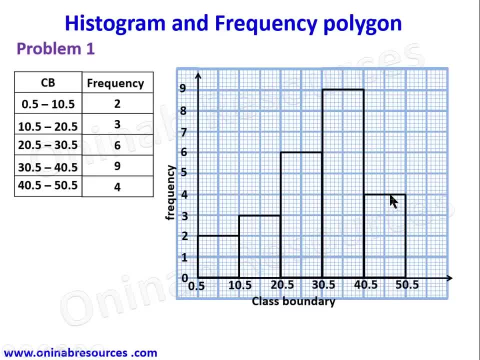 To get the midpoint of 0 and 1, we assume there is a number 0 before 1.. We are going to find the midpoint of 0 and 1.. To get the midpoint of 0 and 1, we assume there is a number 0 before 1.. We are going to find the midpoint of 0 and 1.. 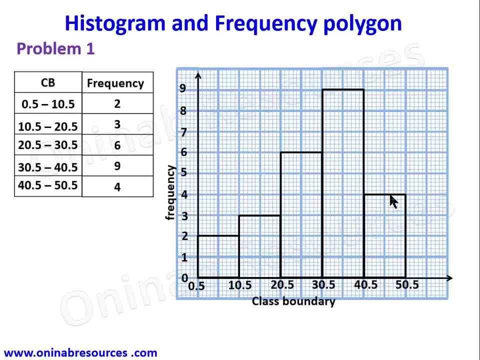 To get the midpoint of 0 and 1, we assume there is a number 0 before 1.. We are going to find the midpoint of 0 and 1.. To get the midpoint of 0 and 1, we assume there is a number 0 before 1.. We are going to find the midpoint of 0 and 1.. 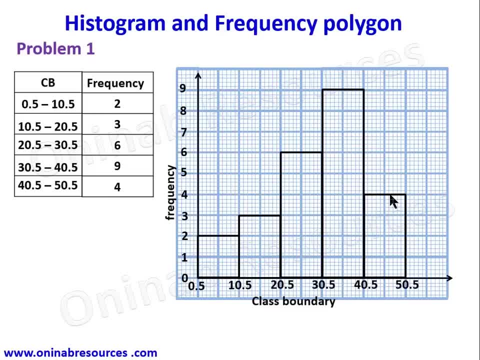 To get the midpoint of 0 and 1, we assume there is a number 0 before 1.. We are going to find the midpoint of 0 and 1.. To get the midpoint of 0 and 1, we assume there is a number 0 before 1.. We are going to find the midpoint of 0 and 1.. 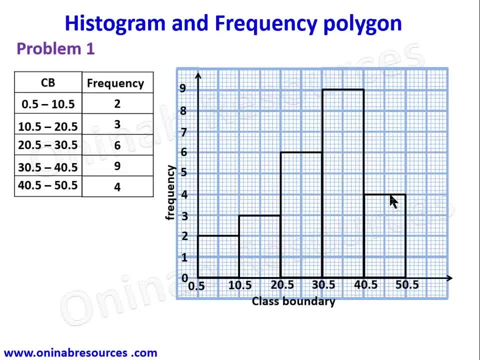 To get the midpoint of 0 and 1, we assume there is a number 0 before 1.. We are going to find the midpoint of 0 and 1.. To get the midpoint of 0 and 1, we assume there is a number 0 before 1.. We are going to find the midpoint of 0 and 1.. 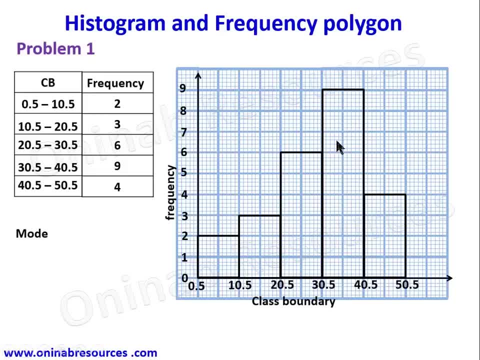 To get the midpoint of 0 and 1, we assume there is a number 0 before 1.. We are going to find the midpoint of 0 and 1.. To get the midpoint of 0 and 1, we assume there is a number 0 before 1.. We are going to find the midpoint of 0 and 1.. 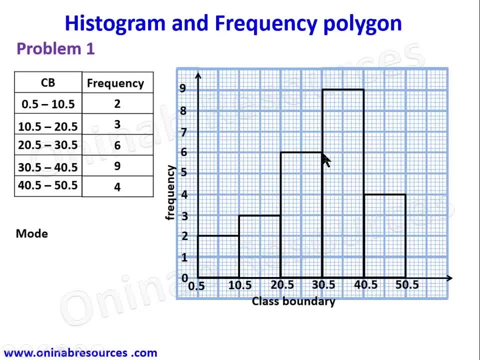 To get the midpoint of 0 and 1, we assume there is a number 0 before 1.. We are going to find the midpoint of 0 and 1.. To get the midpoint of 0 and 1, we assume there is a number 0 before 1.. We are going to find the midpoint of 0 and 1.. 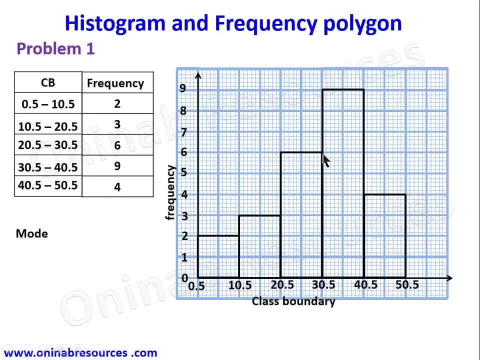 To get the midpoint of 0 and 1, we assume there is a number 0 before 1.. We are going to find the midpoint of 0 and 1.. To get the midpoint of 0 and 1, we assume there is a number 0 before 1.. We are going to find the midpoint of 0 and 1.. 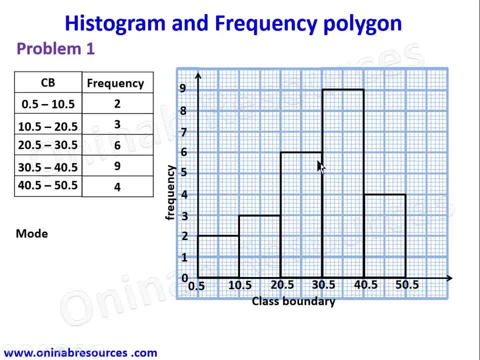 To get the midpoint of 0 and 1, we assume there is a number 0 before 1.. We are going to find the midpoint of 0 and 1.. To get the midpoint of 0 and 1, we assume there is a number 0 before 1.. We are going to find the midpoint of 0 and 1.. 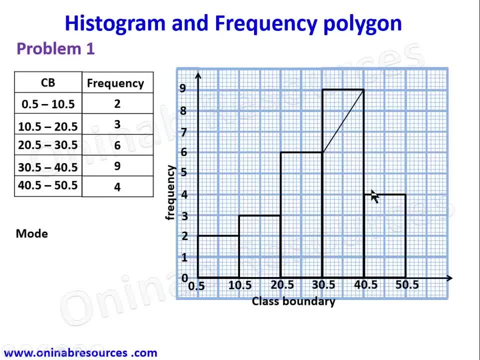 To get the midpoint of 0 and 1, we assume there is a number 0 before 1.. We are going to find the midpoint of 0 and 1.. To get the midpoint of 0 and 1, we assume there is a number 0 before 1.. We are going to find the midpoint of 0 and 1.. 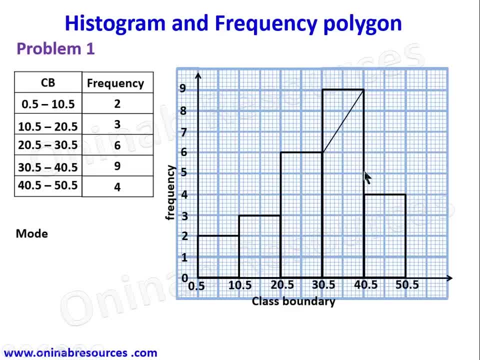 To get the midpoint of 0 and 1, we assume there is a number 0 before 1.. We are going to find the midpoint of 0 and 1.. To get the midpoint of 0 and 1, we assume there is a number 0 before 1.. We are going to find the midpoint of 0 and 1.. 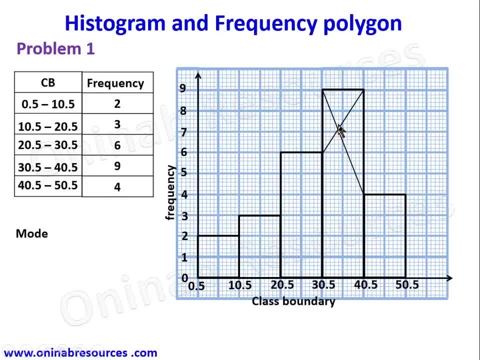 To get the midpoint of 0 and 1, we assume there is a number 0 before 1.. We are going to find the midpoint of 0 and 1.. To get the midpoint of 0 and 1, we assume there is a number 0 before 1.. We are going to find the midpoint of 0 and 1.. 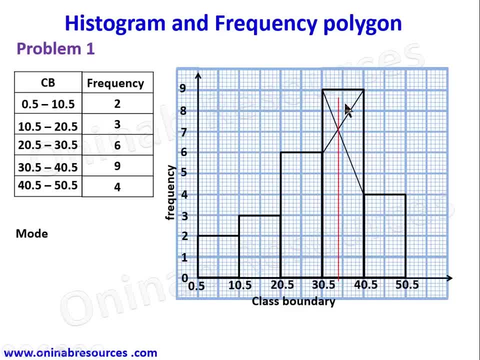 To get the midpoint of 0 and 1, we assume there is a number 0 before 1.. We are going to find the midpoint of 0 and 1.. To get the midpoint of 0 and 1, we assume there is a number 0 before 1.. We are going to find the midpoint of 0 and 1.. 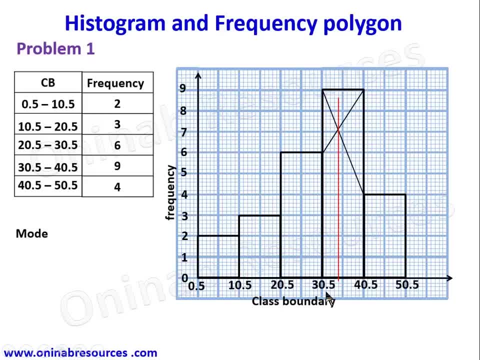 To get the midpoint of 0 and 1, we assume there is a number 0 before 1.. We are going to find the midpoint of 0 and 1.. To get the midpoint of 0 and 1, we assume there is a number 0 before 1.. We are going to find the midpoint of 0 and 1.. 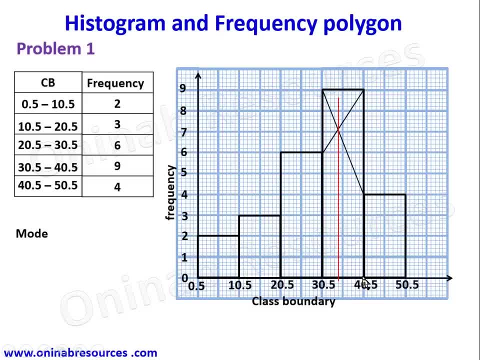 To get the midpoint of 0 and 1, we assume there is a number 0 before 1.. We are going to find the midpoint of 0 and 1.. To get the midpoint of 0 and 1, we assume there is a number 0 before 1.. We are going to find the midpoint of 0 and 1.. 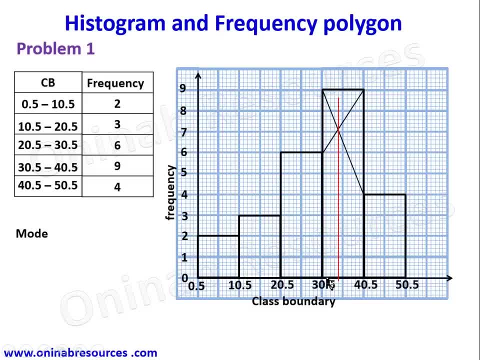 To get the midpoint of 0 and 1, we assume there is a number 0 before 1.. We are going to find the midpoint of 0 and 1.. To get the midpoint of 0 and 1, we assume there is a number 0 before 1.. We are going to find the midpoint of 0 and 1.. 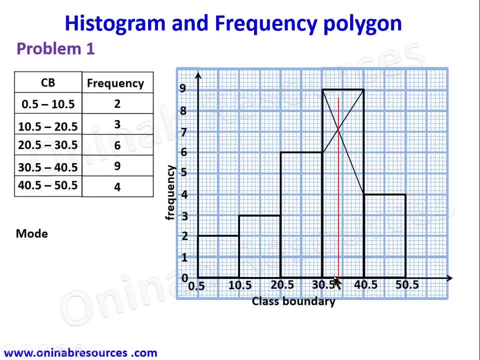 To get the midpoint of 0 and 1, we assume there is a number 0 before 1.. We are going to find the midpoint of 0 and 1.. To get the midpoint of 0 and 1, we assume there is a number 0 before 1.. We are going to find the midpoint of 0 and 1.. 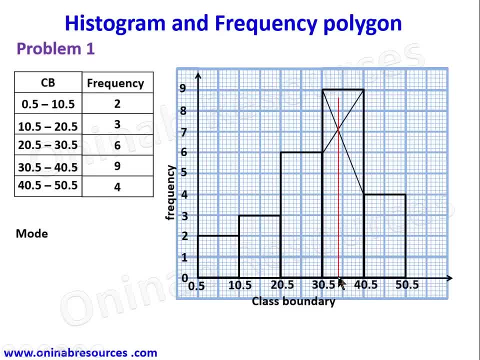 To get the midpoint of 0 and 1, we assume there is a number 0 before 1.. We are going to find the midpoint of 0 and 1.. To get the midpoint of 0 and 1, we assume there is a number 0 before 1.. We are going to find the midpoint of 0 and 1.. 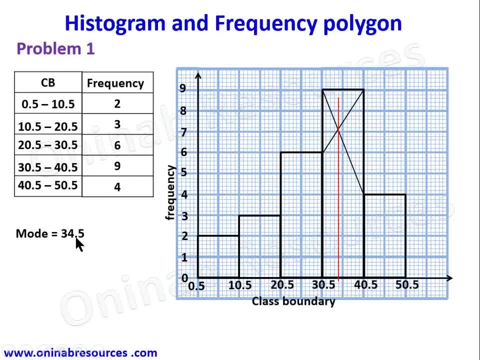 To get the midpoint of 0 and 1, we assume there is a number 0 before 1.. We are going to find the midpoint of 0 and 1.. To get the midpoint of 0 and 1, we assume there is a number 0 before 1.. We are going to find the midpoint of 0 and 1.. 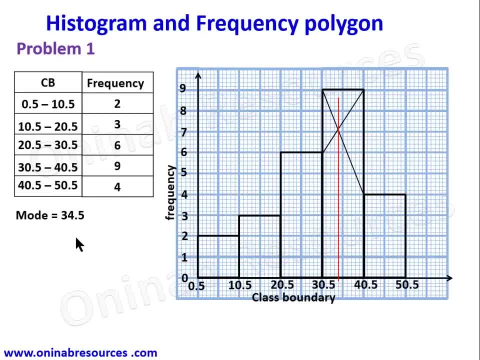 To get the midpoint of 0 and 1, we assume there is a number 0 before 1.. We are going to find the midpoint of 0 and 1.. To get the midpoint of 0 and 1, we assume there is a number 0 before 1.. We are going to find the midpoint of 0 and 1.. 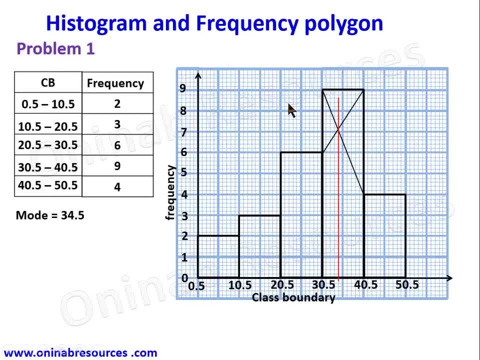 To get the midpoint of 0 and 1, we assume there is a number 0 before 1.. We are going to find the midpoint of 0 and 1.. To get the midpoint of 0 and 1, we assume there is a number 0 before 1.. We are going to find the midpoint of 0 and 1.. 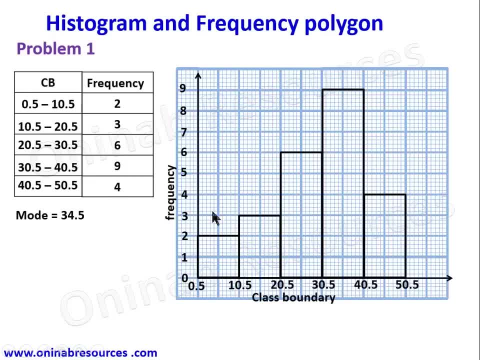 To get the midpoint of 0 and 1, we assume there is a number 0 before 1.. We are going to find the midpoint of 0 and 1.. To get the midpoint of 0 and 1, we assume there is a number 0 before 1.. We are going to find the midpoint of 0 and 1.. 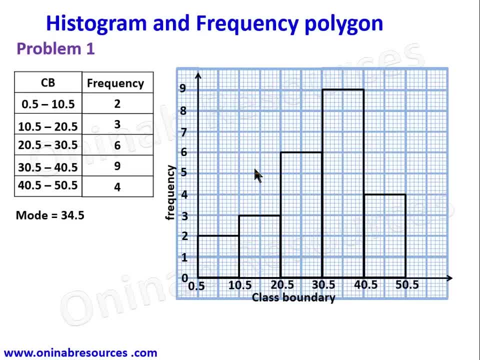 To get the midpoint of 0 and 1, we assume there is a number 0 before 1.. We are going to find the midpoint of 0 and 1.. To get the midpoint of 0 and 1, we assume there is a number 0 before 1.. We are going to find the midpoint of 0 and 1.. 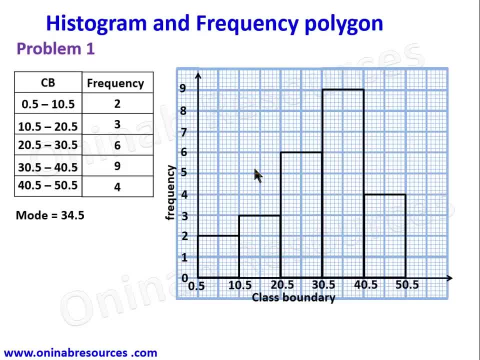 To get the midpoint of 0 and 1, we assume there is a number 0 before 1.. We are going to find the midpoint of 0 and 1.. To get the midpoint of 0 and 1, we assume there is a number 0 before 1.. We are going to find the midpoint of 0 and 1.. 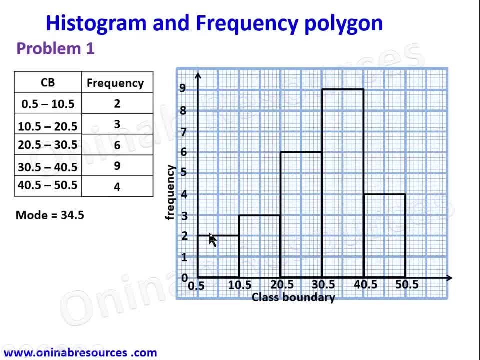 To get the midpoint of 0 and 1, we assume there is a number 0 before 1.. We are going to find the midpoint of 0 and 1.. To get the midpoint of 0 and 1, we assume there is a number 0 before 1.. We are going to find the midpoint of 0 and 1.. 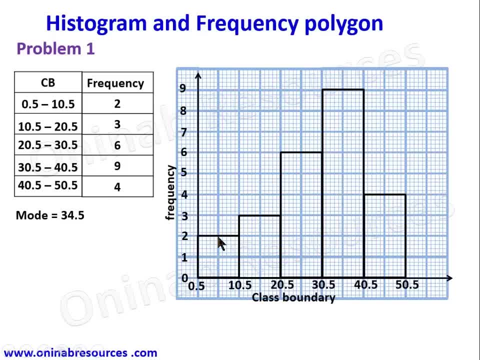 To get the midpoint of 0 and 1, we assume there is a number 0 before 1.. We are going to find the midpoint of 0 and 1.. To get the midpoint of 0 and 1, we assume there is a number 0 before 1.. We are going to find the midpoint of 0 and 1.. 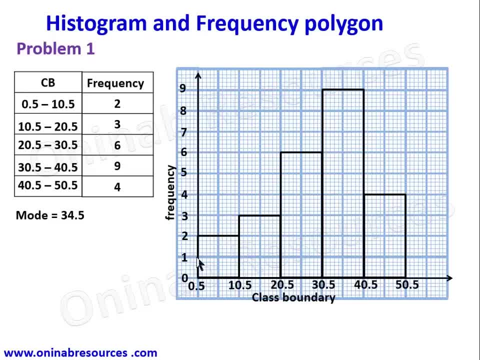 To get the midpoint of 0 and 1, we assume there is a number 0 before 1.. We are going to find the midpoint of 0 and 1.. To get the midpoint of 0 and 1, we assume there is a number 0 before 1.. We are going to find the midpoint of 0 and 1.. 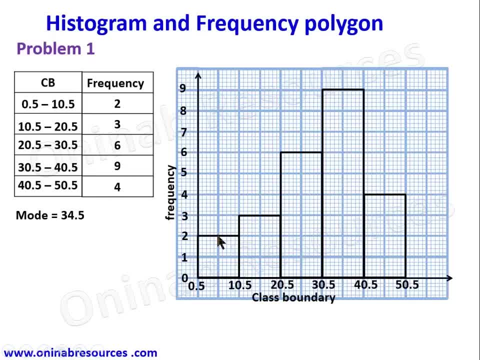 To get the midpoint of 0 and 1, we assume there is a number 0 before 1.. We are going to find the midpoint of 0 and 1.. To get the midpoint of 0 and 1, we assume there is a number 0 before 1.. We are going to find the midpoint of 0 and 1.. 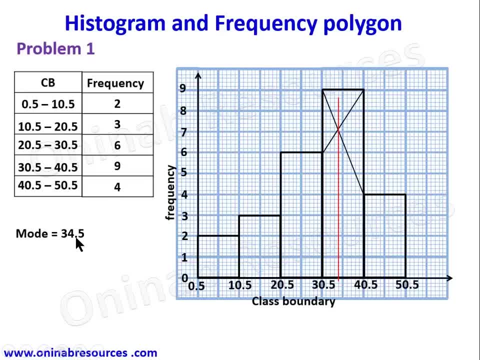 three, four- I also put inside- are left. that when we get to this point of intersection, moving the left efficient one to the right- this is right, this is round and round- are moved to the top of each decline, remains the same. we're saving this, we're saving this. going to the next point of intersection. we're going to translate that to that. 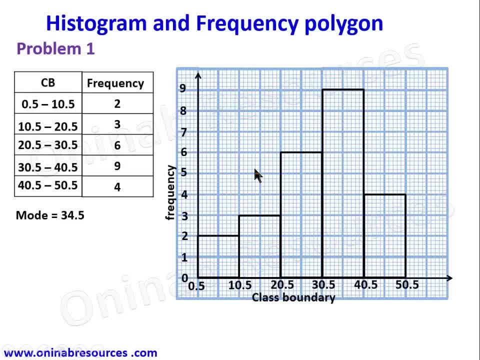 days now to draw the frequency polygon. if you already have an existing histogram of the same distribution, what you do is we get the midway of the height of the bus, then join them together. for the first bar here, this is the midpoint. so we look at the midpoints. the second bar- this is the midpoint, and 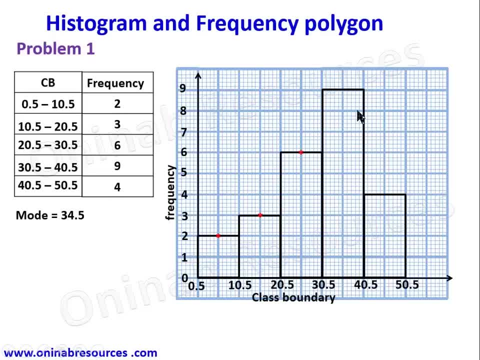 the third bar, the midpoint, the midpoint and the midpoint. here it is a tradition to create an arbitrary midpoints before and after the distribution, since the scale we are using here is 2 centimeters to 10 units. so if you are looking for the midpoint before the class interval, it falls. 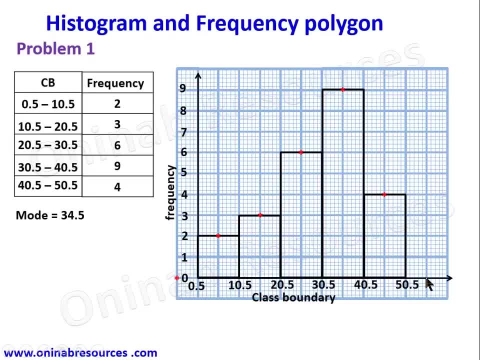 here. if you are looking for the midpoint before the class interval it falls here, after is 1 centimeters, it falls there. so we now joined these midpoints with straight lines. our assumption here is: this is 0, this has frequency 0 and this has frequency 0 by default. since they do not exist, so we assign 0 to them. we now 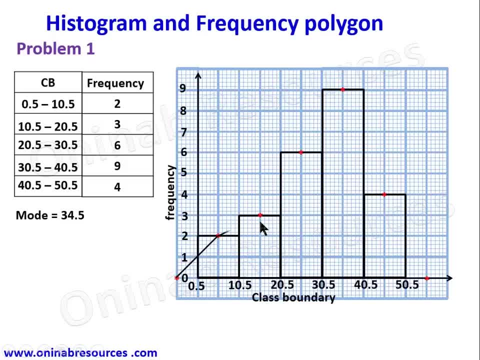 join them. this is joined, joined, joined to the point here. so we joined a final, we join to the end. so this is the frequency polygon, together with the histogram. assuming the histogram is not, there would have gotten something like this. we would have gotten something like this, but 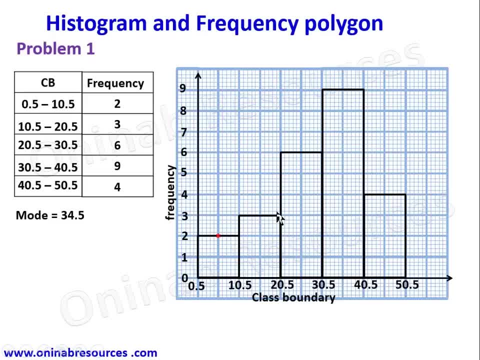 To get the midpoint of 0 and 1, we assume there is a number 0 before 1.. We are going to find the midpoint of 0 and 1.. To get the midpoint of 0 and 1, we assume there is a number 0 before 1.. We are going to find the midpoint of 0 and 1.. 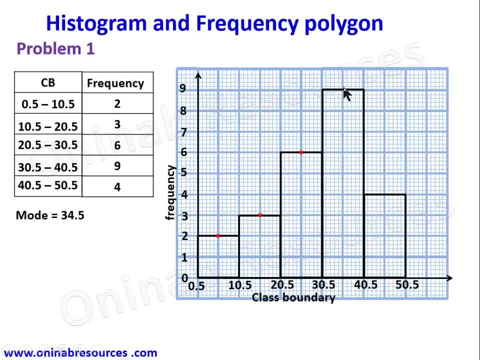 To get the midpoint of 0 and 1, we assume there is a number 0 before 1.. We are going to find the midpoint of 0 and 1.. To get the midpoint of 0 and 1, we assume there is a number 0 before 1.. We are going to find the midpoint of 0 and 1.. 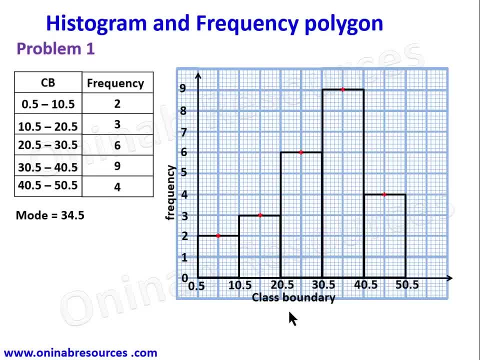 To get the midpoint of 0 and 1, we assume there is a number 0 before 1.. We are going to find the midpoint of 0 and 1.. To get the midpoint of 0 and 1, we assume there is a number 0 before 1.. We are going to find the midpoint of 0 and 1.. 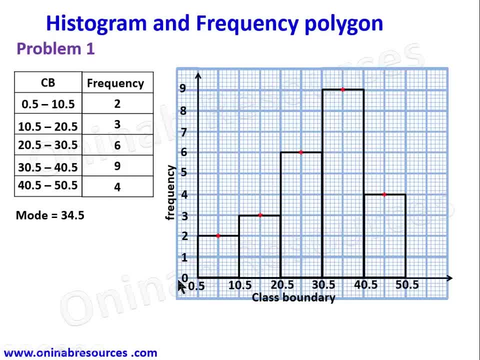 To get the midpoint of 0 and 1, we assume there is a number 0 before 1.. We are going to find the midpoint of 0 and 1.. To get the midpoint of 0 and 1, we assume there is a number 0 before 1.. We are going to find the midpoint of 0 and 1.. 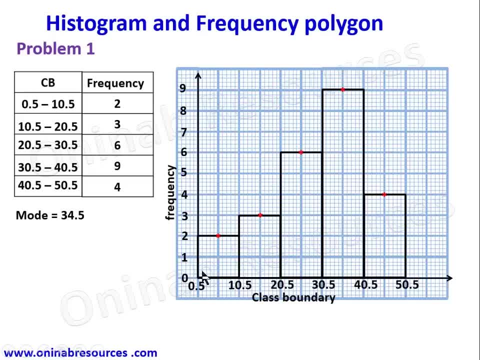 To get the midpoint of 0 and 1, we assume there is a number 0 before 1.. We are going to find the midpoint of 0 and 1.. To get the midpoint of 0 and 1, we assume there is a number 0 before 1.. We are going to find the midpoint of 0 and 1.. 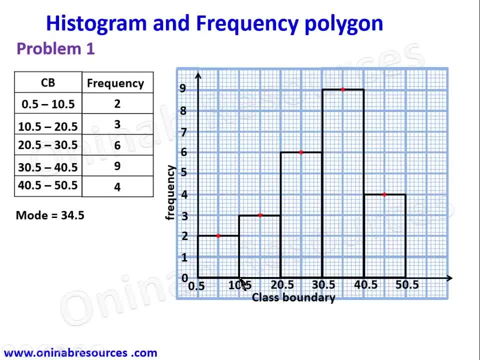 To get the midpoint of 0 and 1, we assume there is a number 0 before 1.. We are going to find the midpoint of 0 and 1.. To get the midpoint of 0 and 1, we assume there is a number 0 before 1.. We are going to find the midpoint of 0 and 1.. 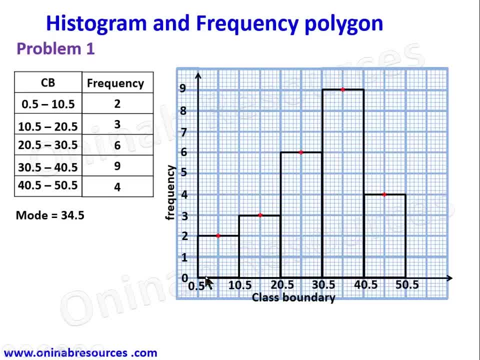 To get the midpoint of 0 and 1, we assume there is a number 0 before 1.. We are going to find the midpoint of 0 and 1.. To get the midpoint of 0 and 1, we assume there is a number 0 before 1.. We are going to find the midpoint of 0 and 1.. 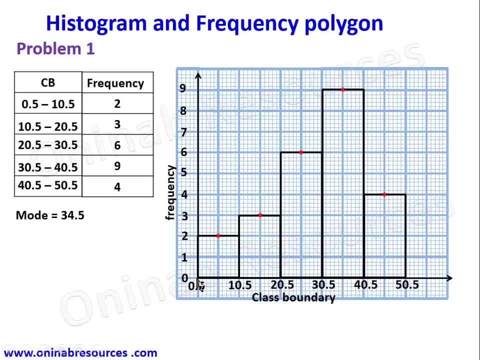 To get the midpoint of 0 and 1, we assume there is a number 0 before 1.. We are going to find the midpoint of 0 and 1.. To get the midpoint of 0 and 1, we assume there is a number 0 before 1.. We are going to find the midpoint of 0 and 1.. 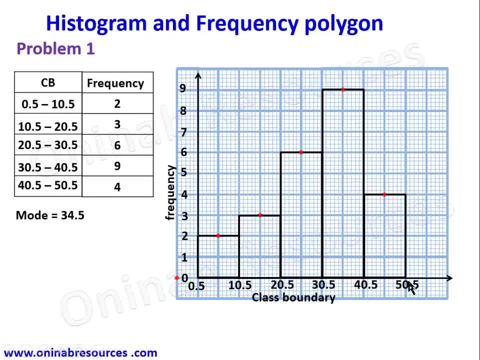 To get the midpoint of 0 and 1, we assume there is a number 0 before 1.. We are going to find the midpoint of 0 and 1.. To get the midpoint of 0 and 1, we assume there is a number 0 before 1.. We are going to find the midpoint of 0 and 1.. 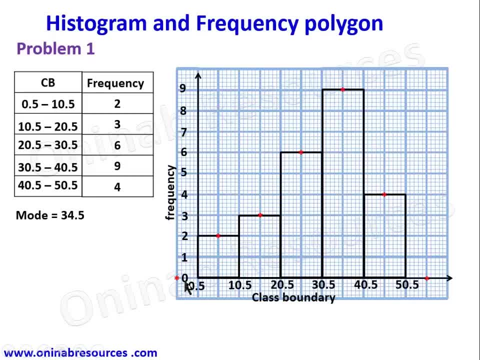 To get the midpoint of 0 and 1, we assume there is a number 0 before 1.. We are going to find the midpoint of 0 and 1.. To get the midpoint of 0 and 1, we assume there is a number 0 before 1.. We are going to find the midpoint of 0 and 1.. 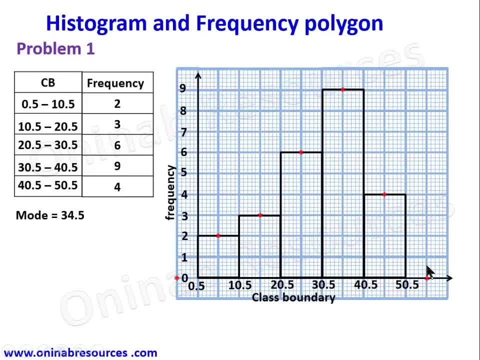 To get the midpoint of 0 and 1, we assume there is a number 0 before 1.. We are going to find the midpoint of 0 and 1.. To get the midpoint of 0 and 1, we assume there is a number 0 before 1.. We are going to find the midpoint of 0 and 1.. 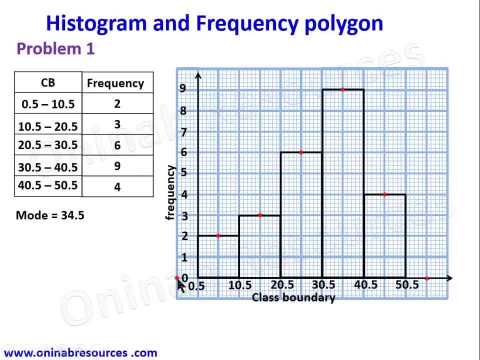 To get the midpoint of 0 and 1, we assume there is a number 0 before 1.. We are going to find the midpoint of 0 and 1.. To get the midpoint of 0 and 1, we assume there is a number 0 before 1.. We are going to find the midpoint of 0 and 1.. 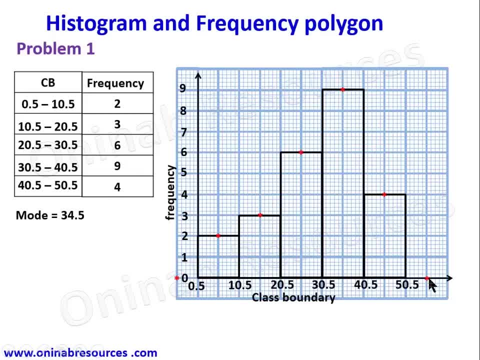 To get the midpoint of 0 and 1, we assume there is a number 0 before 1.. We are going to find the midpoint of 0 and 1.. To get the midpoint of 0 and 1, we assume there is a number 0 before 1.. We are going to find the midpoint of 0 and 1.. 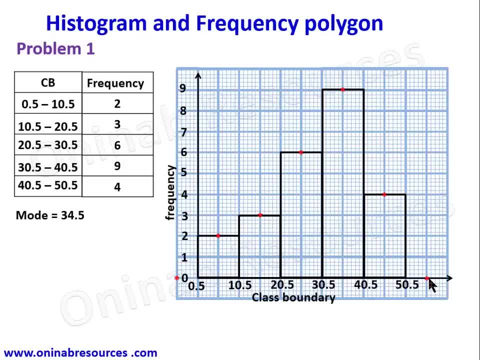 To get the midpoint of 0 and 1, we assume there is a number 0 before 1.. We are going to find the midpoint of 0 and 1.. To get the midpoint of 0 and 1, we assume there is a number 0 before 1.. We are going to find the midpoint of 0 and 1.. 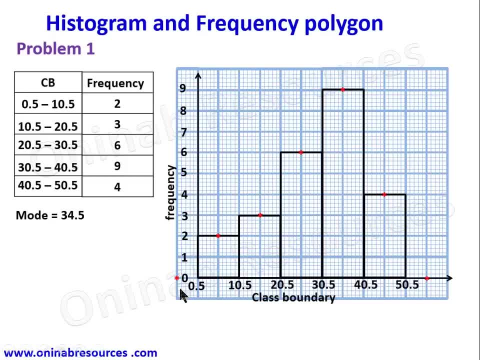 To get the midpoint of 0 and 1, we assume there is a number 0 before 1.. We are going to find the midpoint of 0 and 1.. To get the midpoint of 0 and 1, we assume there is a number 0 before 1.. We are going to find the midpoint of 0 and 1.. 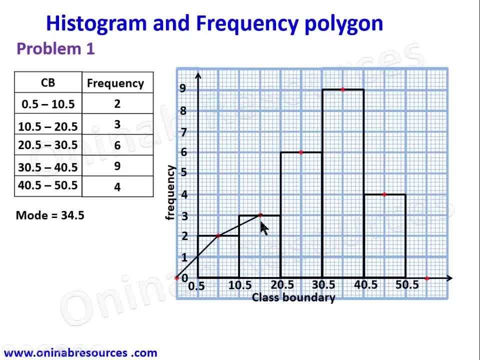 To get the midpoint of 0 and 1, we assume there is a number 0 before 1.. We are going to find the midpoint of 0 and 1.. To get the midpoint of 0 and 1, we assume there is a number 0 before 1.. We are going to find the midpoint of 0 and 1.. 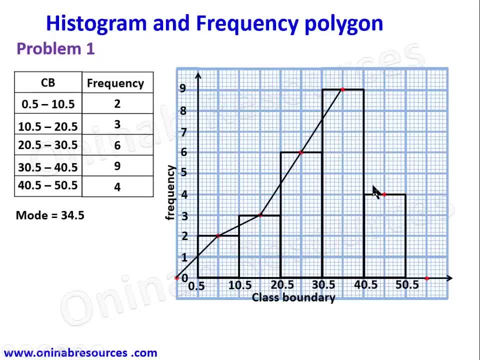 To get the midpoint of 0 and 1, we assume there is a number 0 before 1.. We are going to find the midpoint of 0 and 1.. To get the midpoint of 0 and 1, we assume there is a number 0 before 1.. We are going to find the midpoint of 0 and 1.. 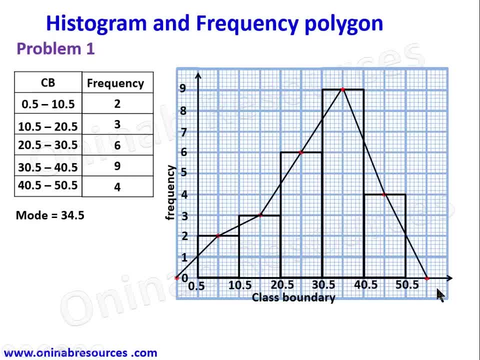 To get the midpoint of 0 and 1, we assume there is a number 0 before 1.. We are going to find the midpoint of 0 and 1.. To get the midpoint of 0 and 1, we assume there is a number 0 before 1.. We are going to find the midpoint of 0 and 1.. 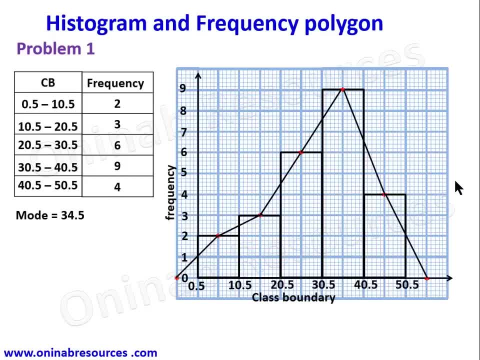 To get the midpoint of 0 and 1, we assume there is a number 0 before 1.. We are going to find the midpoint of 0 and 1.. To get the midpoint of 0 and 1, we assume there is a number 0 before 1.. We are going to find the midpoint of 0 and 1.. 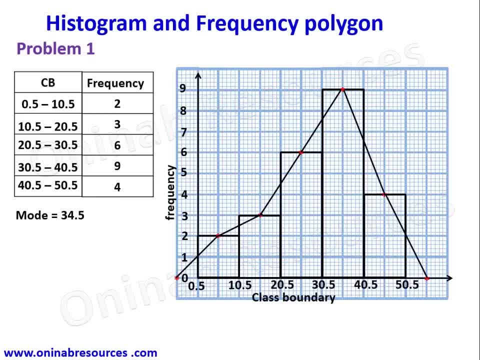 To get the midpoint of 0 and 1, we assume there is a number 0 before 1.. We are going to find the midpoint of 0 and 1.. To get the midpoint of 0 and 1, we assume there is a number 0 before 1.. We are going to find the midpoint of 0 and 1.. 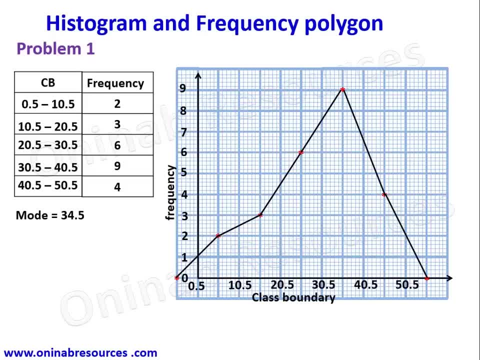 To get the midpoint of 0 and 1, we assume there is a number 0 before 1.. We are going to find the midpoint of 0 and 1.. To get the midpoint of 0 and 1, we assume there is a number 0 before 1.. We are going to find the midpoint of 0 and 1.. 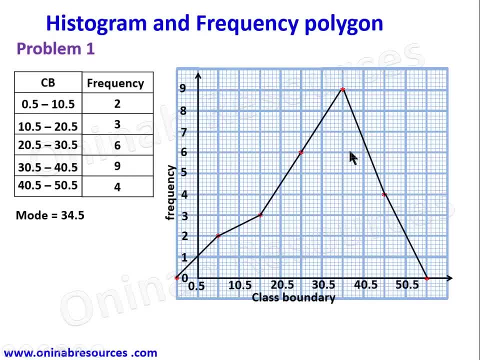 To get the midpoint of 0 and 1, we assume there is a number 0 before 1.. We are going to find the midpoint of 0 and 1.. To get the midpoint of 0 and 1, we assume there is a number 0 before 1.. We are going to find the midpoint of 0 and 1.. 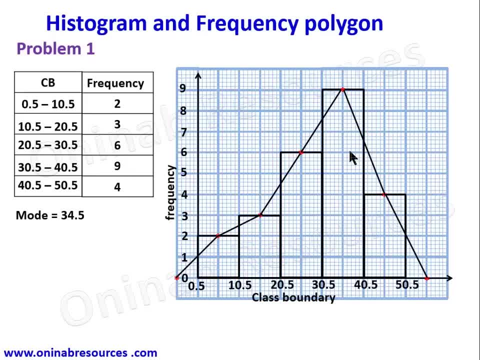 To get the midpoint of 0 and 1, we assume there is a number 0 before 1.. We are going to find the midpoint of 0 and 1.. To get the midpoint of 0 and 1, we assume there is a number 0 before 1.. We are going to find the midpoint of 0 and 1.. 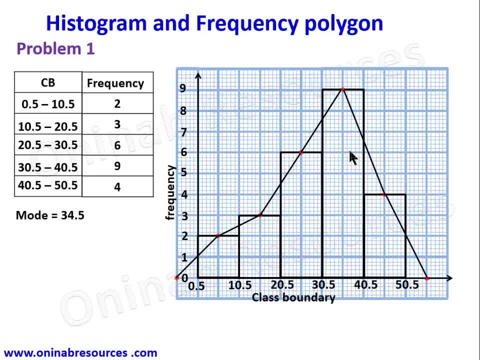 To get the midpoint of 0 and 1, we assume there is a number 0 before 1.. We are going to find the midpoint of 0 and 1.. To get the midpoint of 0 and 1, we assume there is a number 0 before 1.. We are going to find the midpoint of 0 and 1.. 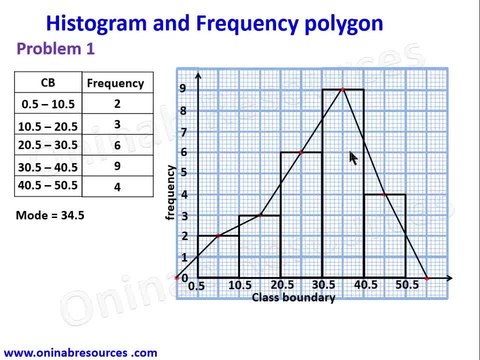 To get the midpoint of 0 and 1, we assume there is a number 0 before 1.. We are going to find the midpoint of 0 and 1.. To get the midpoint of 0 and 1, we assume there is a number 0 before 1.. We are going to find the midpoint of 0 and 1.. 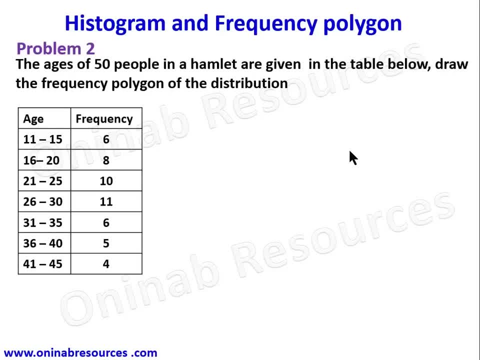 To get the midpoint of 0 and 1, we assume there is a number 0 before 1.. We are going to find the midpoint of 0 and 1.. To get the midpoint of 0 and 1, we assume there is a number 0 before 1.. We are going to find the midpoint of 0 and 1.. 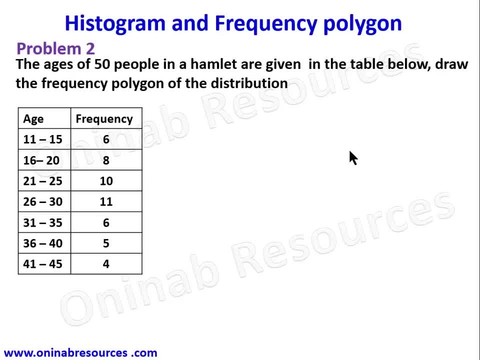 To get the midpoint of 0 and 1, we assume there is a number 0 before 1.. We are going to find the midpoint of 0 and 1.. To get the midpoint of 0 and 1, we assume there is a number 0 before 1.. We are going to find the midpoint of 0 and 1.. 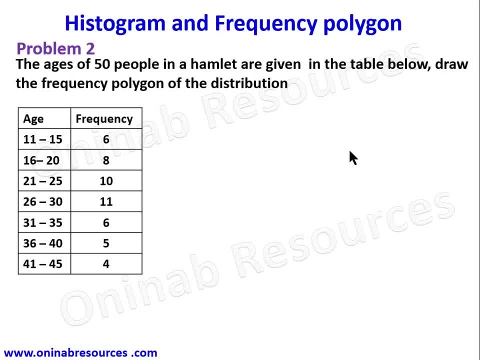 To get the midpoint of 0 and 1, we assume there is a number 0 before 1.. We are going to find the midpoint of 0 and 1.. To get the midpoint of 0 and 1, we assume there is a number 0 before 1.. We are going to find the midpoint of 0 and 1.. 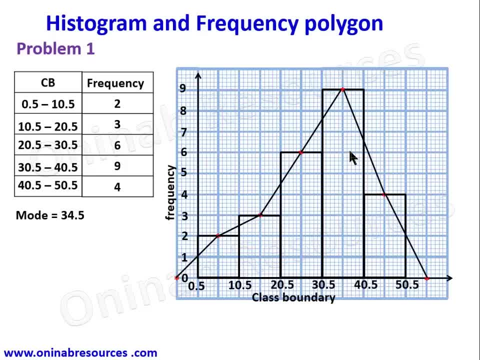 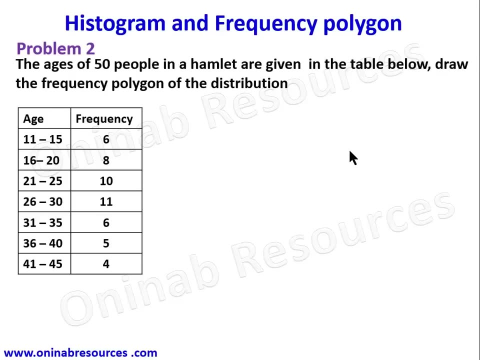 since the histogram is there, we have it together with the histogram, and that is the end of solution to problem one. we go to problem two from here. for problem two, the ages of 50 people in a hamlet are given in the table below. draw the frequency polygon of the distribution. so here we are drawing only the frequency. 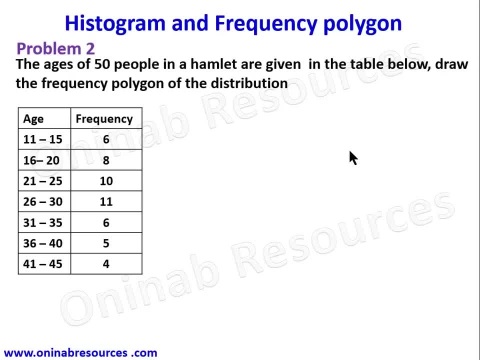 polygon. so we are going to learn how to get this. by default, the frequency polygon is the mid-value on the horizontal axis and the frequency on the vertical axis. so we are going to create additional column to this table to give us the class made fun. so the class made volume will be adding the lower class interval to the upper class interval. 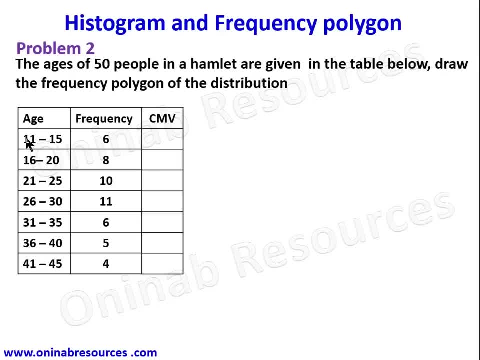 to the upper class interval and then interval and divide your sum by 2 to get the mid value for each of the class intervals. we then start from the first class interval. 11 plus 15 gives 26, divided by 2 gives 13, and 16 plus 20 divided by 2 gives 18, 21 plus 25 divided. 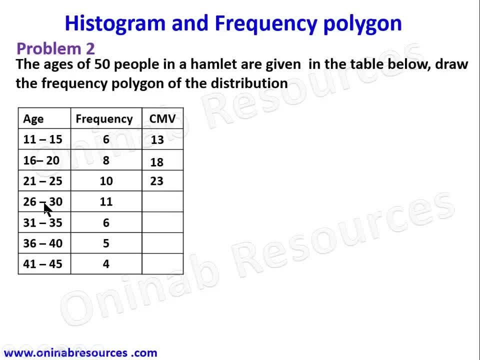 by 2 gives 23. 26 plus 30 divided by 2 gives 28, 31 plus 35 divided by 2 gives 33. 36 plus 40 divided by 2 gives 38 and finally, 41 plus 45 divided by 2 gives a. 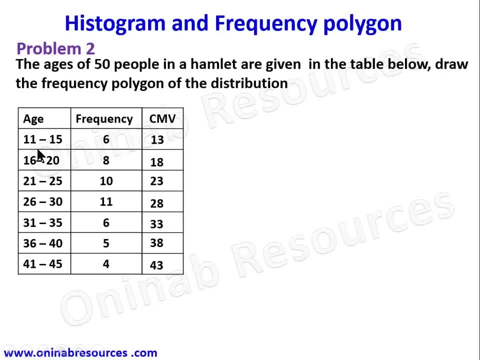 43. this are the class mid value for the class E in class E in E class intervals. so we are going to be drawing the frequency polygon using the classmate value on the horizontal axis and the frequencies on the vertical axis. so we bring in our graph. 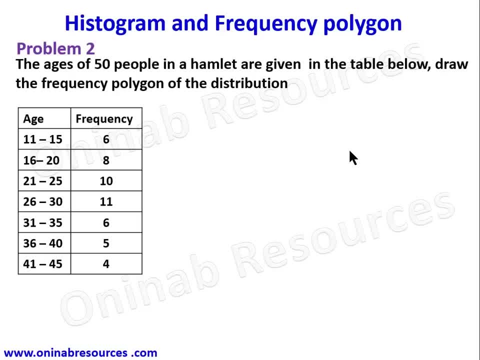 To get the midpoint of 0 and 1, we assume there is a number 0 before 1.. We are going to find the midpoint of 0 and 1.. To get the midpoint of 0 and 1, we assume there is a number 0 before 1.. We are going to find the midpoint of 0 and 1.. 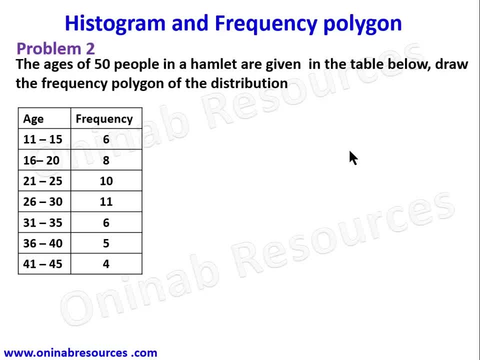 To get the midpoint of 0 and 1, we assume there is a number 0 before 1.. We are going to find the midpoint of 0 and 1.. To get the midpoint of 0 and 1, we assume there is a number 0 before 1.. We are going to find the midpoint of 0 and 1.. 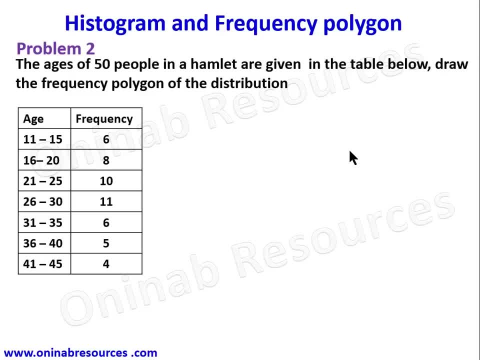 To get the midpoint of 0 and 1, we assume there is a number 0 before 1.. We are going to find the midpoint of 0 and 1.. To get the midpoint of 0 and 1, we assume there is a number 0 before 1.. We are going to find the midpoint of 0 and 1.. 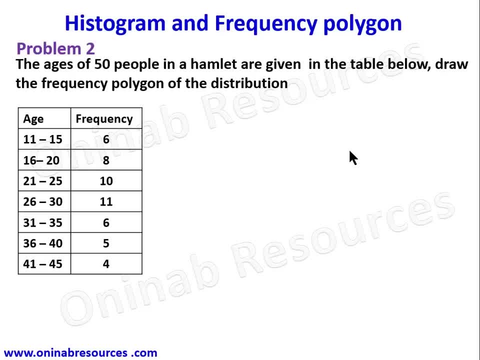 To get the midpoint of 0 and 1, we assume there is a number 0 before 1.. We are going to find the midpoint of 0 and 1.. To get the midpoint of 0 and 1, we assume there is a number 0 before 1.. We are going to find the midpoint of 0 and 1.. 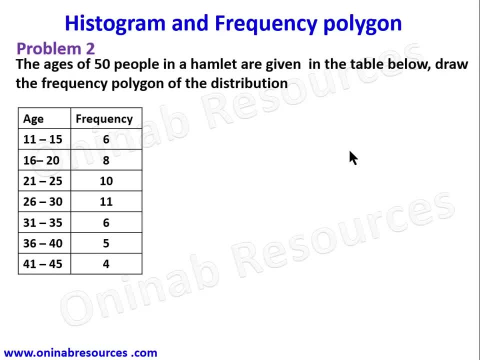 To get the midpoint of 0 and 1, we assume there is a number 0 before 1.. We are going to find the midpoint of 0 and 1.. To get the midpoint of 0 and 1, we assume there is a number 0 before 1.. We are going to find the midpoint of 0 and 1.. 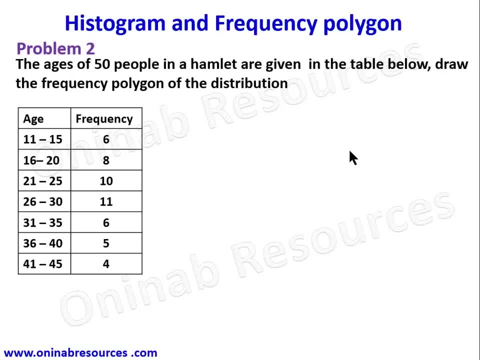 To get the midpoint of 0 and 1, we assume there is a number 0 before 1.. We are going to find the midpoint of 0 and 1.. To get the midpoint of 0 and 1, we assume there is a number 0 before 1.. We are going to find the midpoint of 0 and 1.. 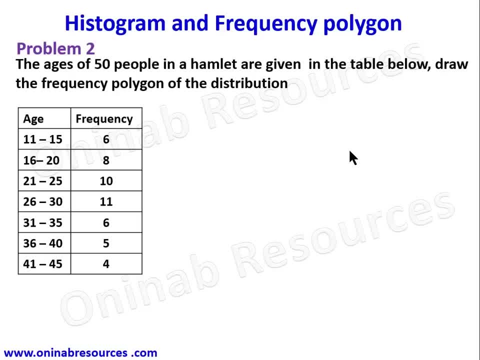 To get the midpoint of 0 and 1, we assume there is a number 0 before 1.. We are going to find the midpoint of 0 and 1.. To get the midpoint of 0 and 1, we assume there is a number 0 before 1.. We are going to find the midpoint of 0 and 1.. 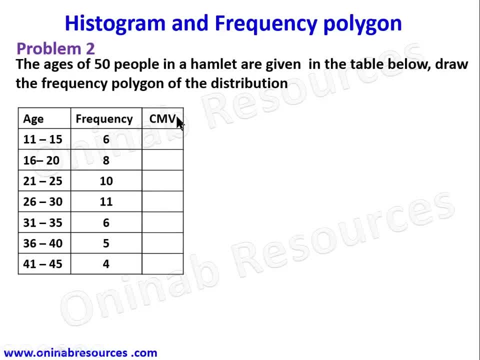 To get the midpoint of 0 and 1, we assume there is a number 0 before 1.. We are going to find the midpoint of 0 and 1.. To get the midpoint of 0 and 1, we assume there is a number 0 before 1.. We are going to find the midpoint of 0 and 1.. 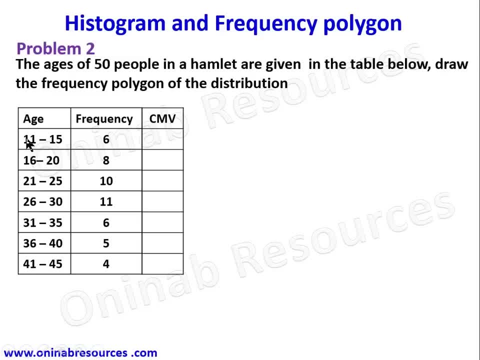 To get the midpoint of 0 and 1, we assume there is a number 0 before 1.. We are going to find the midpoint of 0 and 1.. To get the midpoint of 0 and 1, we assume there is a number 0 before 1.. We are going to find the midpoint of 0 and 1.. 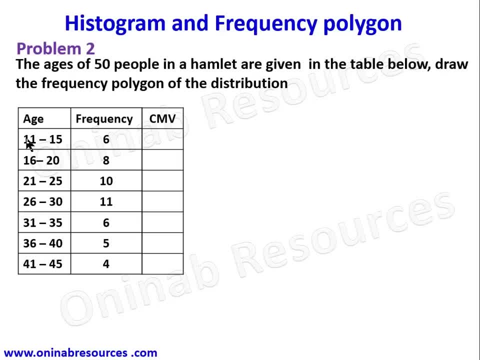 To get the midpoint of 0 and 1, we assume there is a number 0 before 1.. We are going to find the midpoint of 0 and 1.. To get the midpoint of 0 and 1, we assume there is a number 0 before 1.. We are going to find the midpoint of 0 and 1.. 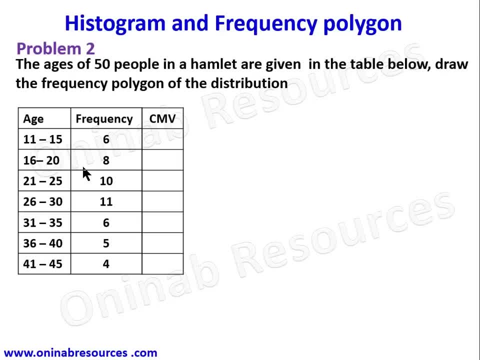 To get the midpoint of 0 and 1, we assume there is a number 0 before 1.. We are going to find the midpoint of 0 and 1.. To get the midpoint of 0 and 1, we assume there is a number 0 before 1.. We are going to find the midpoint of 0 and 1.. 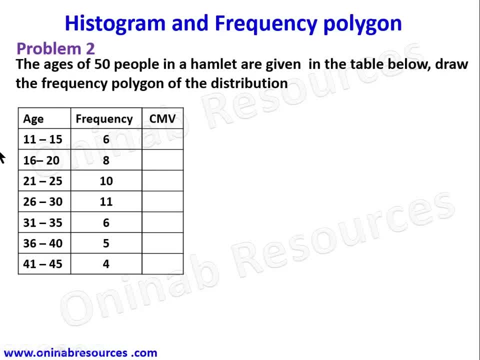 To get the midpoint of 0 and 1, we assume there is a number 0 before 1.. We are going to find the midpoint of 0 and 1.. To get the midpoint of 0 and 1, we assume there is a number 0 before 1.. We are going to find the midpoint of 0 and 1.. 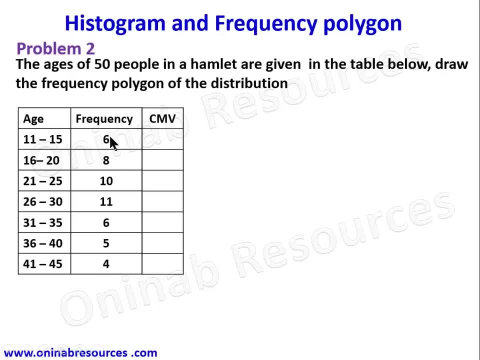 To get the midpoint of 0 and 1, we assume there is a number 0 before 1.. We are going to find the midpoint of 0 and 1.. To get the midpoint of 0 and 1, we assume there is a number 0 before 1.. We are going to find the midpoint of 0 and 1.. 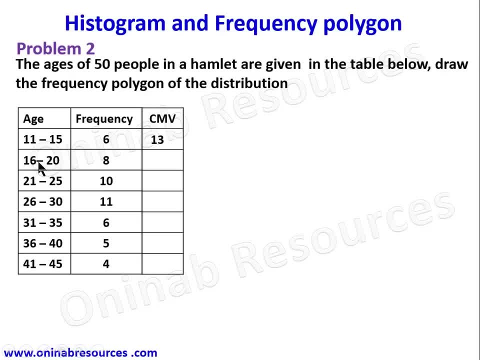 To get the midpoint of 0 and 1, we assume there is a number 0 before 1.. We are going to find the midpoint of 0 and 1.. To get the midpoint of 0 and 1, we assume there is a number 0 before 1.. We are going to find the midpoint of 0 and 1.. 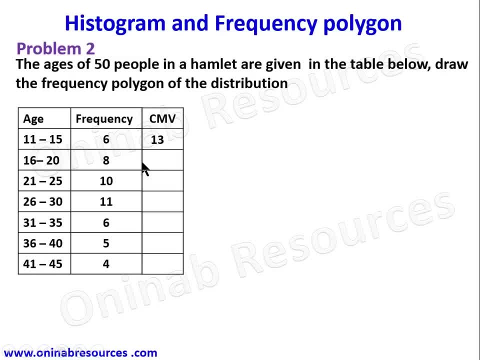 To get the midpoint of 0 and 1, we assume there is a number 0 before 1.. We are going to find the midpoint of 0 and 1.. To get the midpoint of 0 and 1, we assume there is a number 0 before 1.. We are going to find the midpoint of 0 and 1.. 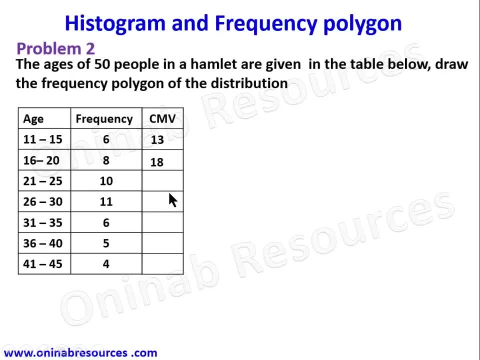 To get the midpoint of 0 and 1, we assume there is a number 0 before 1.. We are going to find the midpoint of 0 and 1.. To get the midpoint of 0 and 1, we assume there is a number 0 before 1.. We are going to find the midpoint of 0 and 1.. 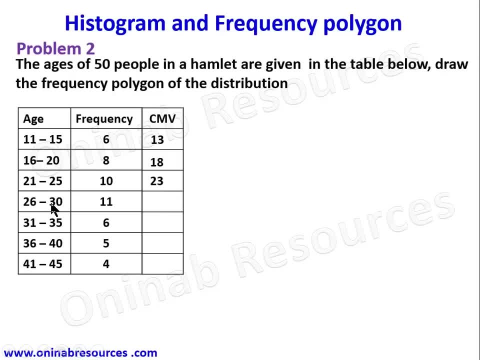 To get the midpoint of 0 and 1, we assume there is a number 0 before 1.. We are going to find the midpoint of 0 and 1.. To get the midpoint of 0 and 1, we assume there is a number 0 before 1.. We are going to find the midpoint of 0 and 1.. 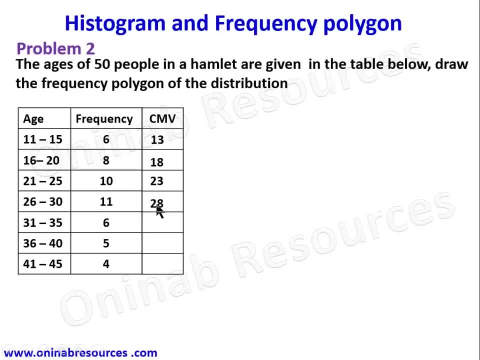 To get the midpoint of 0 and 1, we assume there is a number 0 before 1.. We are going to find the midpoint of 0 and 1.. To get the midpoint of 0 and 1, we assume there is a number 0 before 1.. We are going to find the midpoint of 0 and 1.. 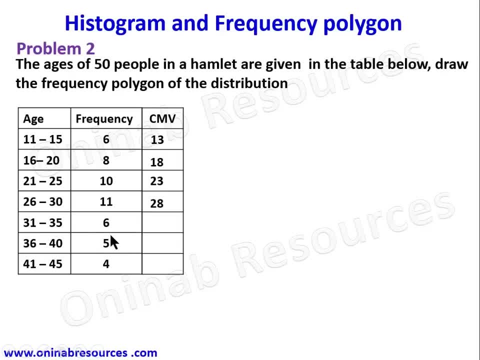 To get the midpoint of 0 and 1, we assume there is a number 0 before 1.. We are going to find the midpoint of 0 and 1.. To get the midpoint of 0 and 1, we assume there is a number 0 before 1.. We are going to find the midpoint of 0 and 1.. 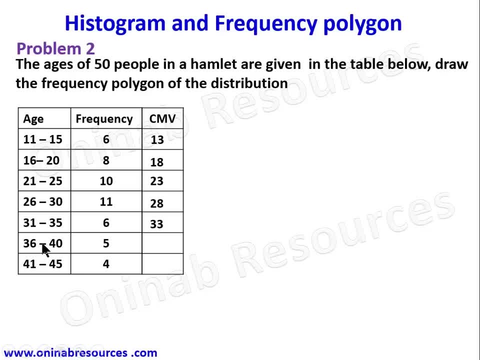 To get the midpoint of 0 and 1, we assume there is a number 0 before 1.. We are going to find the midpoint of 0 and 1.. To get the midpoint of 0 and 1, we assume there is a number 0 before 1.. We are going to find the midpoint of 0 and 1.. 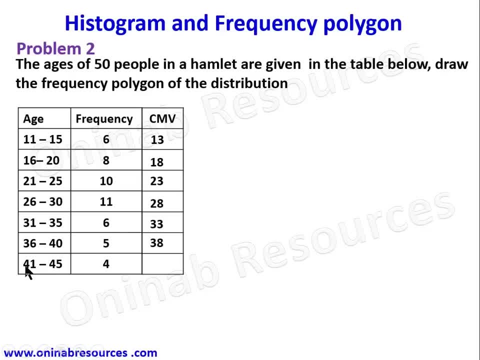 To get the midpoint of 0 and 1, we assume there is a number 0 before 1.. We are going to find the midpoint of 0 and 1.. To get the midpoint of 0 and 1, we assume there is a number 0 before 1.. We are going to find the midpoint of 0 and 1.. 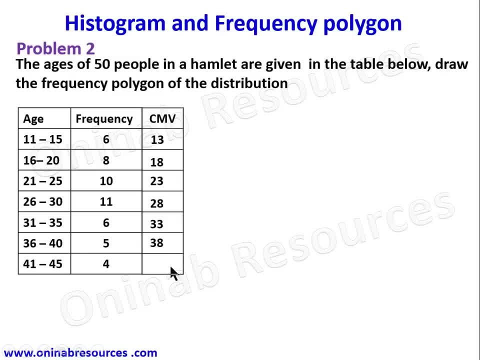 To get the midpoint of 0 and 1, we assume there is a number 0 before 1.. We are going to find the midpoint of 0 and 1.. To get the midpoint of 0 and 1, we assume there is a number 0 before 1.. We are going to find the midpoint of 0 and 1.. 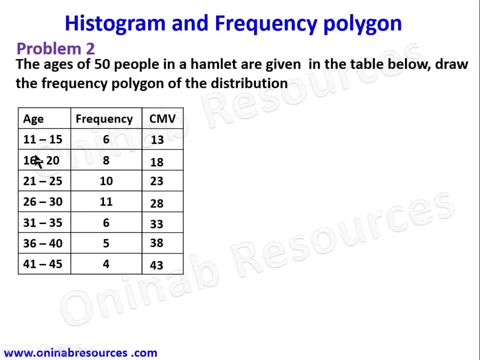 To get the midpoint of 0 and 1, we assume there is a number 0 before 1.. We are going to find the midpoint of 0 and 1.. To get the midpoint of 0 and 1, we assume there is a number 0 before 1.. We are going to find the midpoint of 0 and 1.. 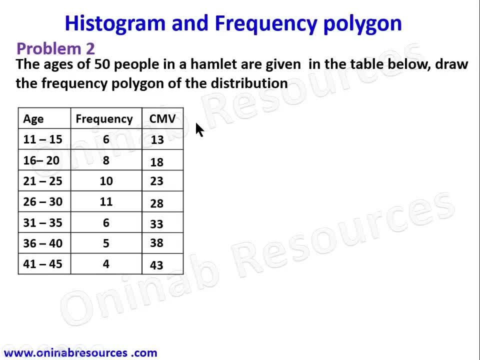 To get the midpoint of 0 and 1, we assume there is a number 0 before 1.. We are going to find the midpoint of 0 and 1.. To get the midpoint of 0 and 1, we assume there is a number 0 before 1.. We are going to find the midpoint of 0 and 1.. 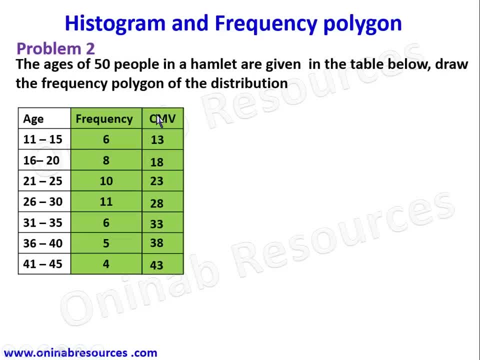 To get the midpoint of 0 and 1, we assume there is a number 0 before 1.. We are going to find the midpoint of 0 and 1.. To get the midpoint of 0 and 1, we assume there is a number 0 before 1.. We are going to find the midpoint of 0 and 1.. 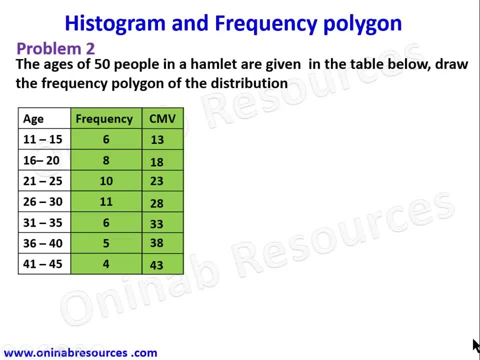 To get the midpoint of 0 and 1, we assume there is a number 0 before 1.. We are going to find the midpoint of 0 and 1.. To get the midpoint of 0 and 1, we assume there is a number 0 before 1.. We are going to find the midpoint of 0 and 1.. 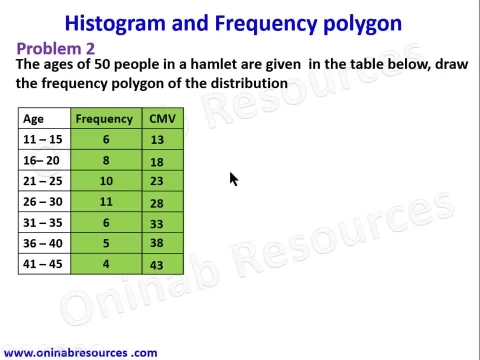 To get the midpoint of 0 and 1, we assume there is a number 0 before 1.. We are going to find the midpoint of 0 and 1.. To get the midpoint of 0 and 1, we assume there is a number 0 before 1.. We are going to find the midpoint of 0 and 1.. 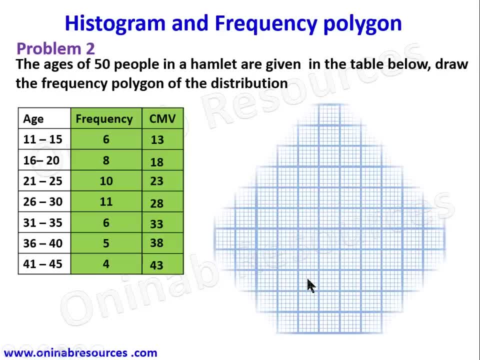 To get the midpoint of 0 and 1, we assume there is a number 0 before 1.. We are going to find the midpoint of 0 and 1.. To get the midpoint of 0 and 1, we assume there is a number 0 before 1.. We are going to find the midpoint of 0 and 1.. 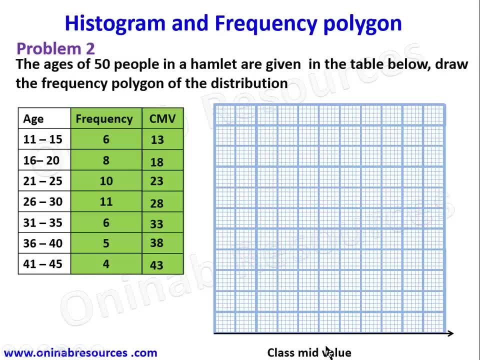 so, from the graph, this is the classmate value and this is the frequency for the classmate value. we are starting from 13, 18, 23, 28, 33, 38 and 43, and here we have it as 0, 1, 2, 3, 4, 5, 6, 7, 8, 9, 10 and 11, since the highest frequency is 11. so we stop. 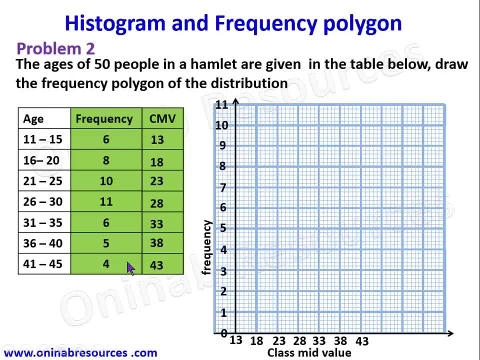 at 11. so we now create an arbitrary mid value before the class interval and after the class interval so that the frequency polygon can be joined together and those class mid value will be assigned zero. so if you look at this now, this is a sequence of addition of 5, 5, 5. so if you subtract 5 from 13, that will 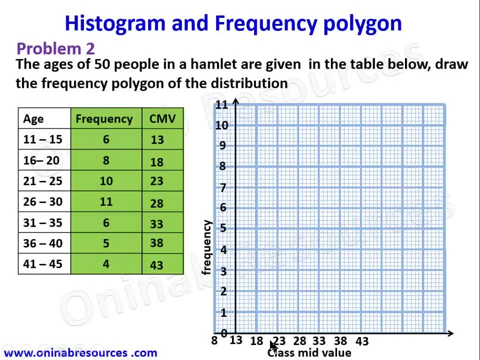 give us 8, so the mid value before 13 is 8, and we add 43 to 5, we give us 48, which gives the mid value of the arbitrary class interval after the last class interval. now we start with this: this is 0. we assign it 0 for 13. the frequency is 6, so we have the point. 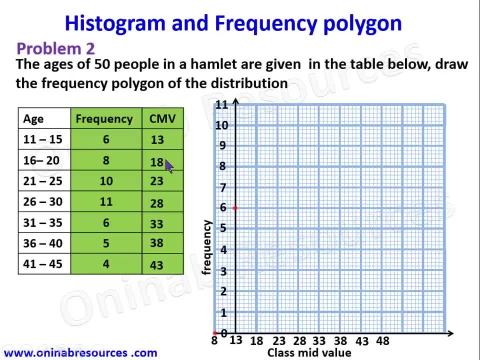 here. for 18, the frequency is 8, so we have the point here. and for 23, the frequency is 10, the frequency is 10. here for 28, 28, the frequency is 11, so we have it as 11 here, 13 with straight lines. so from here we have this, this, from here to this, from here to 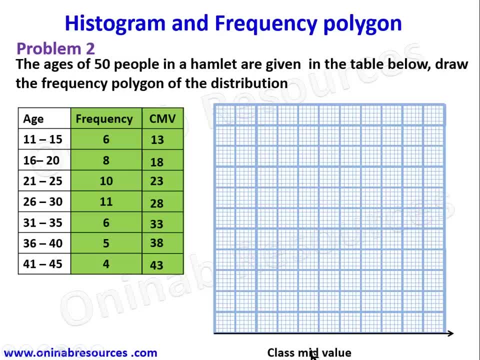 To get the midpoint of 0 and 1, we assume there is a number 0 before 1.. We are going to find the midpoint of 0 and 1.. To get the midpoint of 0 and 1, we assume there is a number 0 before 1.. We are going to find the midpoint of 0 and 1.. 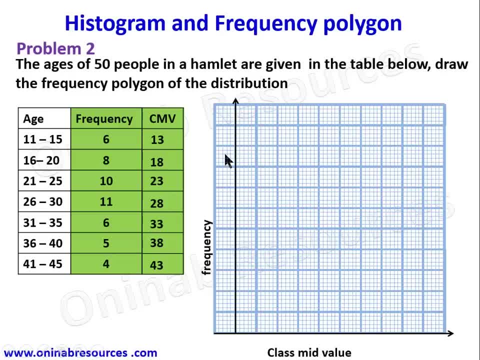 To get the midpoint of 0 and 1, we assume there is a number 0 before 1.. We are going to find the midpoint of 0 and 1.. To get the midpoint of 0 and 1, we assume there is a number 0 before 1.. We are going to find the midpoint of 0 and 1.. 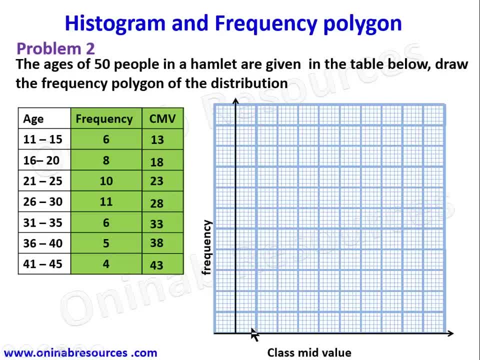 To get the midpoint of 0 and 1, we assume there is a number 0 before 1.. We are going to find the midpoint of 0 and 1.. To get the midpoint of 0 and 1, we assume there is a number 0 before 1.. We are going to find the midpoint of 0 and 1.. 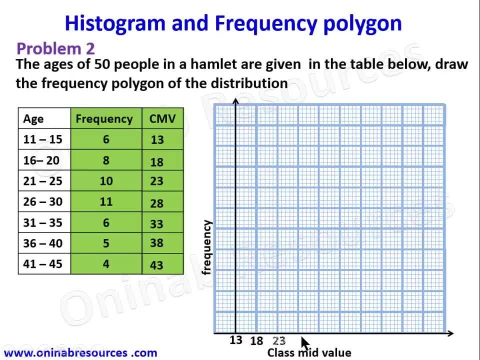 To get the midpoint of 0 and 1, we assume there is a number 0 before 1.. We are going to find the midpoint of 0 and 1.. To get the midpoint of 0 and 1, we assume there is a number 0 before 1.. We are going to find the midpoint of 0 and 1.. 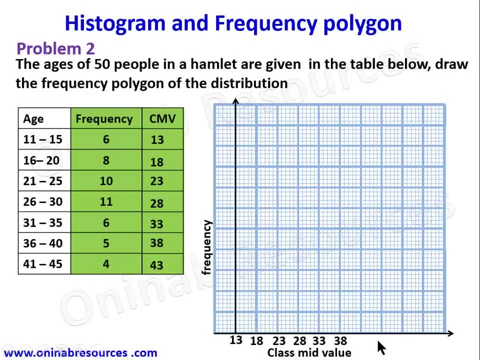 To get the midpoint of 0 and 1, we assume there is a number 0 before 1.. We are going to find the midpoint of 0 and 1.. To get the midpoint of 0 and 1, we assume there is a number 0 before 1.. We are going to find the midpoint of 0 and 1.. 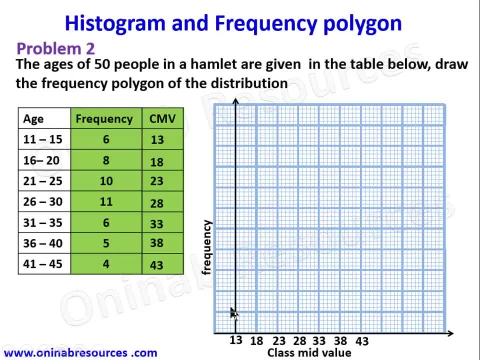 To get the midpoint of 0 and 1, we assume there is a number 0 before 1.. We are going to find the midpoint of 0 and 1.. To get the midpoint of 0 and 1, we assume there is a number 0 before 1.. We are going to find the midpoint of 0 and 1.. 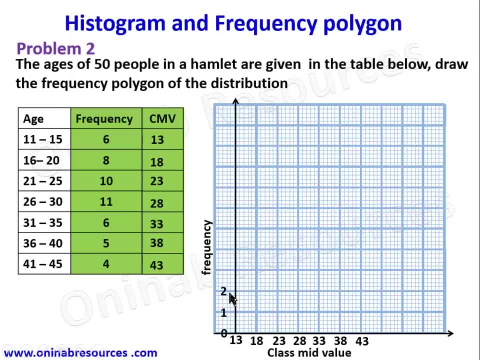 To get the midpoint of 0 and 1, we assume there is a number 0 before 1.. We are going to find the midpoint of 0 and 1.. To get the midpoint of 0 and 1, we assume there is a number 0 before 1.. We are going to find the midpoint of 0 and 1.. 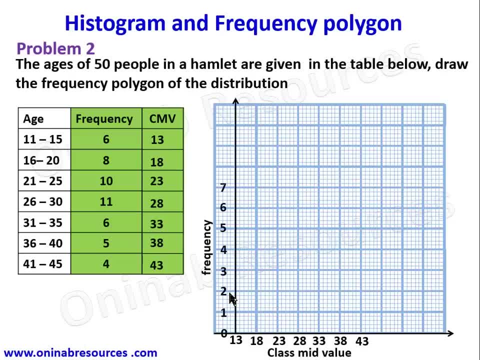 To get the midpoint of 0 and 1, we assume there is a number 0 before 1.. We are going to find the midpoint of 0 and 1.. To get the midpoint of 0 and 1, we assume there is a number 0 before 1.. We are going to find the midpoint of 0 and 1.. 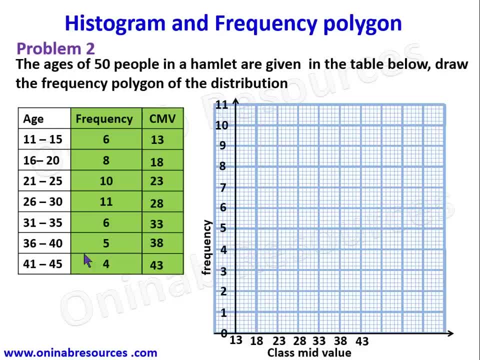 To get the midpoint of 0 and 1, we assume there is a number 0 before 1.. We are going to find the midpoint of 0 and 1.. To get the midpoint of 0 and 1, we assume there is a number 0 before 1.. We are going to find the midpoint of 0 and 1.. 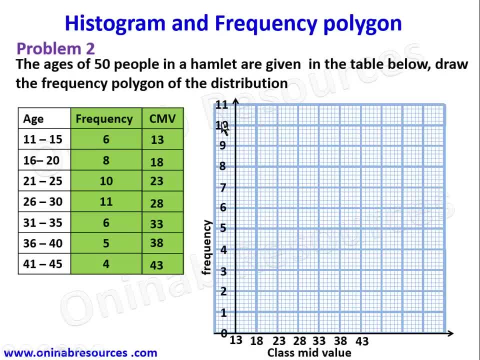 To get the midpoint of 0 and 1, we assume there is a number 0 before 1.. We are going to find the midpoint of 0 and 1.. To get the midpoint of 0 and 1, we assume there is a number 0 before 1.. We are going to find the midpoint of 0 and 1.. 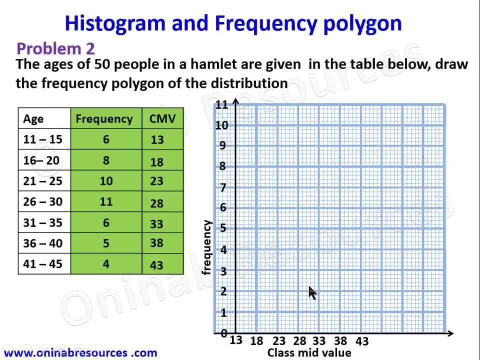 To get the midpoint of 0 and 1, we assume there is a number 0 before 1.. We are going to find the midpoint of 0 and 1.. To get the midpoint of 0 and 1, we assume there is a number 0 before 1.. We are going to find the midpoint of 0 and 1.. 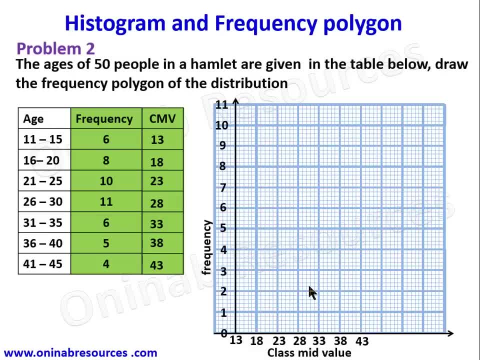 To get the midpoint of 0 and 1, we assume there is a number 0 before 1.. We are going to find the midpoint of 0 and 1.. To get the midpoint of 0 and 1, we assume there is a number 0 before 1.. We are going to find the midpoint of 0 and 1.. 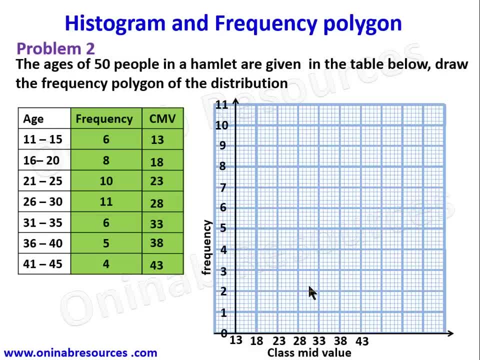 To get the midpoint of 0 and 1, we assume there is a number 0 before 1.. We are going to find the midpoint of 0 and 1.. To get the midpoint of 0 and 1, we assume there is a number 0 before 1.. We are going to find the midpoint of 0 and 1.. 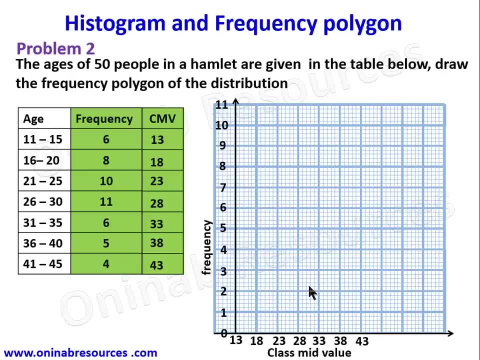 To get the midpoint of 0 and 1, we assume there is a number 0 before 1.. We are going to find the midpoint of 0 and 1.. To get the midpoint of 0 and 1, we assume there is a number 0 before 1.. We are going to find the midpoint of 0 and 1.. 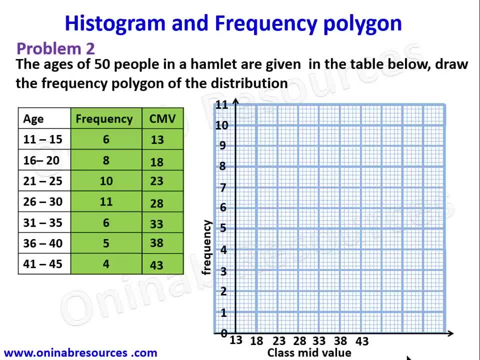 To get the midpoint of 0 and 1, we assume there is a number 0 before 1.. We are going to find the midpoint of 0 and 1.. To get the midpoint of 0 and 1, we assume there is a number 0 before 1.. We are going to find the midpoint of 0 and 1.. 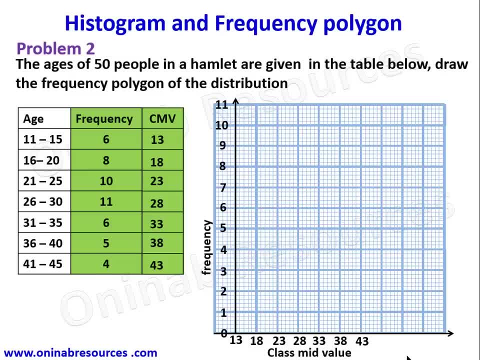 To get the midpoint of 0 and 1, we assume there is a number 0 before 1.. We are going to find the midpoint of 0 and 1.. To get the midpoint of 0 and 1, we assume there is a number 0 before 1.. We are going to find the midpoint of 0 and 1.. 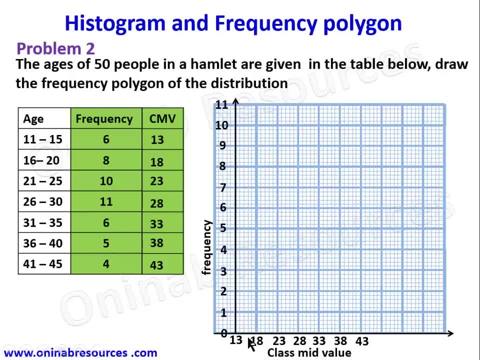 To get the midpoint of 0 and 1, we assume there is a number 0 before 1.. We are going to find the midpoint of 0 and 1.. To get the midpoint of 0 and 1, we assume there is a number 0 before 1.. We are going to find the midpoint of 0 and 1.. 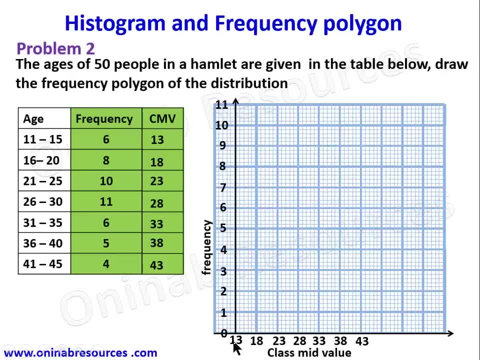 To get the midpoint of 0 and 1, we assume there is a number 0 before 1.. We are going to find the midpoint of 0 and 1.. To get the midpoint of 0 and 1, we assume there is a number 0 before 1.. We are going to find the midpoint of 0 and 1.. 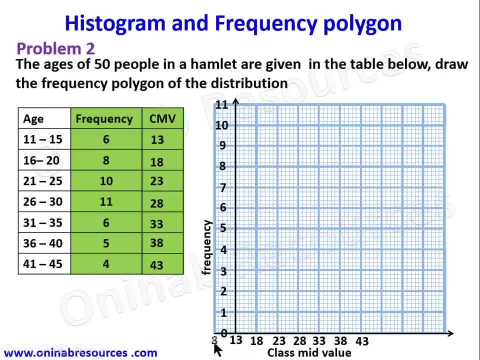 To get the midpoint of 0 and 1, we assume there is a number 0 before 1.. We are going to find the midpoint of 0 and 1.. To get the midpoint of 0 and 1, we assume there is a number 0 before 1.. We are going to find the midpoint of 0 and 1.. 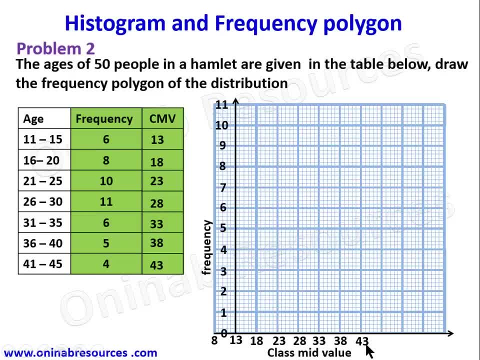 To get the midpoint of 0 and 1, we assume there is a number 0 before 1.. We are going to find the midpoint of 0 and 1.. To get the midpoint of 0 and 1, we assume there is a number 0 before 1.. We are going to find the midpoint of 0 and 1.. 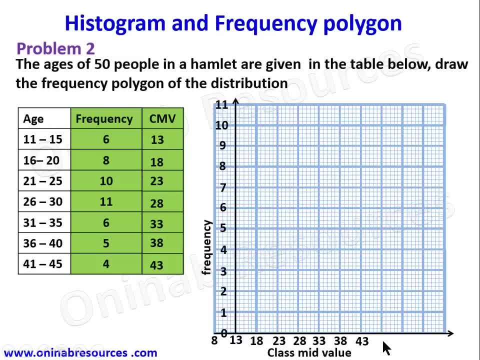 To get the midpoint of 0 and 1, we assume there is a number 0 before 1.. We are going to find the midpoint of 0 and 1.. To get the midpoint of 0 and 1, we assume there is a number 0 before 1.. We are going to find the midpoint of 0 and 1.. 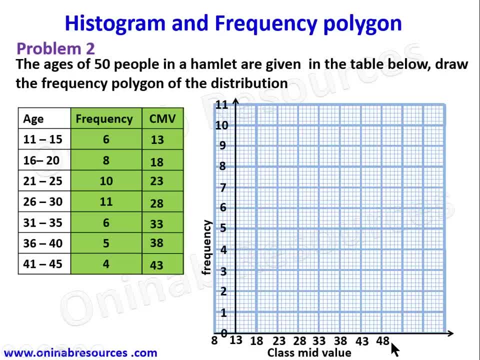 To get the midpoint of 0 and 1, we assume there is a number 0 before 1.. We are going to find the midpoint of 0 and 1.. To get the midpoint of 0 and 1, we assume there is a number 0 before 1.. We are going to find the midpoint of 0 and 1.. 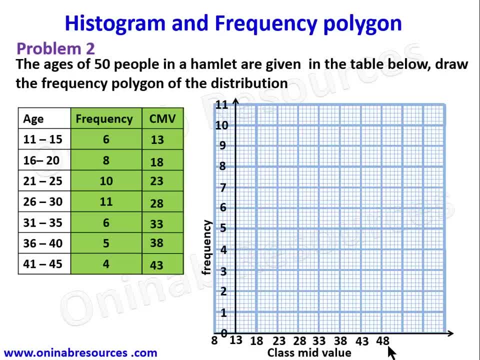 To get the midpoint of 0 and 1, we assume there is a number 0 before 1.. We are going to find the midpoint of 0 and 1.. To get the midpoint of 0 and 1, we assume there is a number 0 before 1.. We are going to find the midpoint of 0 and 1.. 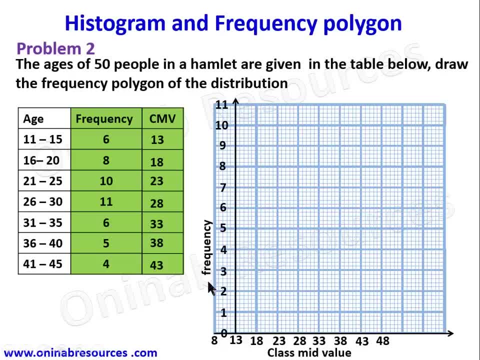 To get the midpoint of 0 and 1, we assume there is a number 0 before 1.. We are going to find the midpoint of 0 and 1.. To get the midpoint of 0 and 1, we assume there is a number 0 before 1.. We are going to find the midpoint of 0 and 1.. 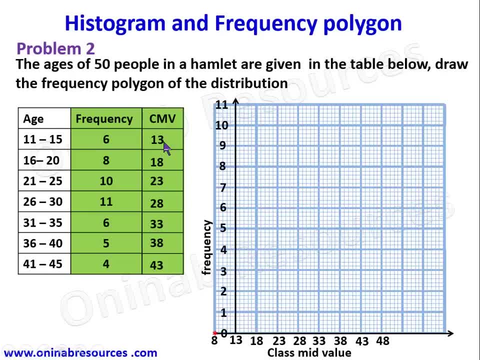 To get the midpoint of 0 and 1, we assume there is a number 0 before 1.. We are going to find the midpoint of 0 and 1.. To get the midpoint of 0 and 1, we assume there is a number 0 before 1.. We are going to find the midpoint of 0 and 1.. 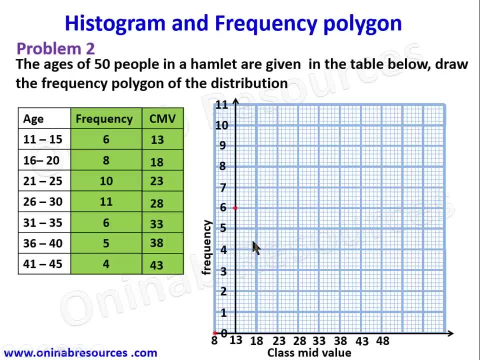 To get the midpoint of 0 and 1, we assume there is a number 0 before 1.. We are going to find the midpoint of 0 and 1.. To get the midpoint of 0 and 1, we assume there is a number 0 before 1.. We are going to find the midpoint of 0 and 1.. 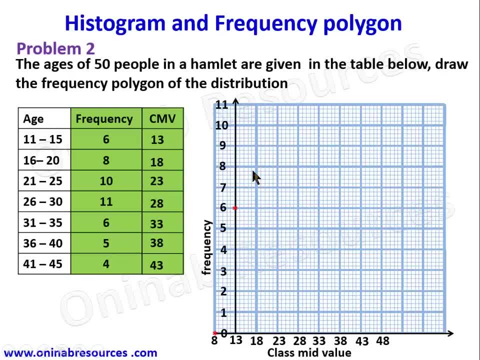 To get the midpoint of 0 and 1, we assume there is a number 0 before 1.. We are going to find the midpoint of 0 and 1.. To get the midpoint of 0 and 1, we assume there is a number 0 before 1.. We are going to find the midpoint of 0 and 1.. 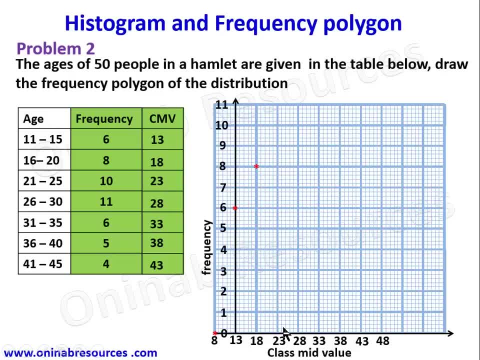 To get the midpoint of 0 and 1, we assume there is a number 0 before 1.. We are going to find the midpoint of 0 and 1.. To get the midpoint of 0 and 1, we assume there is a number 0 before 1.. We are going to find the midpoint of 0 and 1.. 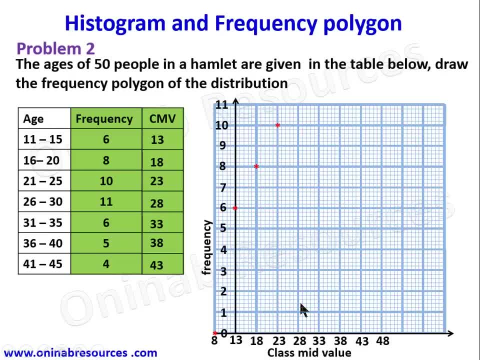 To get the midpoint of 0 and 1, we assume there is a number 0 before 1.. We are going to find the midpoint of 0 and 1.. To get the midpoint of 0 and 1, we assume there is a number 0 before 1.. We are going to find the midpoint of 0 and 1.. 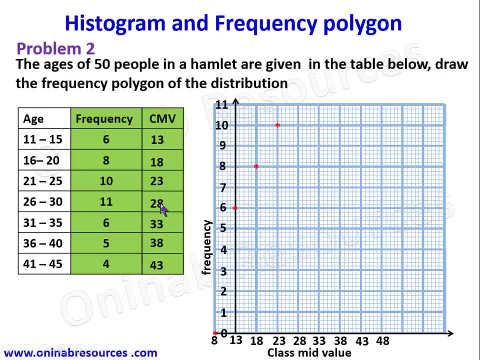 To get the midpoint of 0 and 1, we assume there is a number 0 before 1.. We are going to find the midpoint of 0 and 1.. To get the midpoint of 0 and 1, we assume there is a number 0 before 1.. We are going to find the midpoint of 0 and 1.. 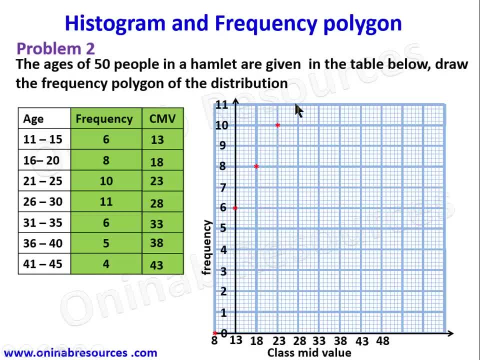 To get the midpoint of 0 and 1, we assume there is a number 0 before 1.. We are going to find the midpoint of 0 and 1.. To get the midpoint of 0 and 1, we assume there is a number 0 before 1.. We are going to find the midpoint of 0 and 1.. 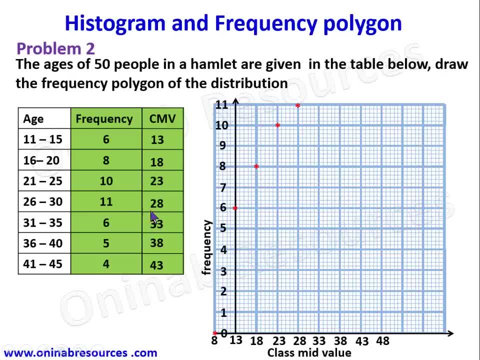 To get the midpoint of 0 and 1, we assume there is a number 0 before 1.. We are going to find the midpoint of 0 and 1.. To get the midpoint of 0 and 1, we assume there is a number 0 before 1.. We are going to find the midpoint of 0 and 1.. 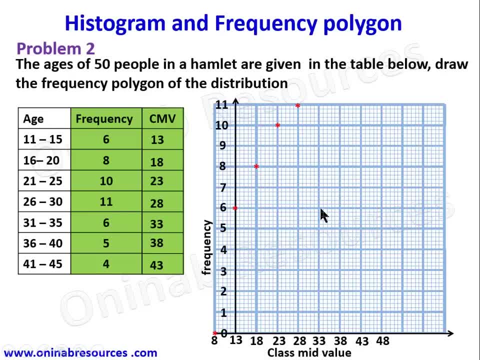 To get the midpoint of 0 and 1, we assume there is a number 0 before 1.. We are going to find the midpoint of 0 and 1.. To get the midpoint of 0 and 1, we assume there is a number 0 before 1.. We are going to find the midpoint of 0 and 1.. 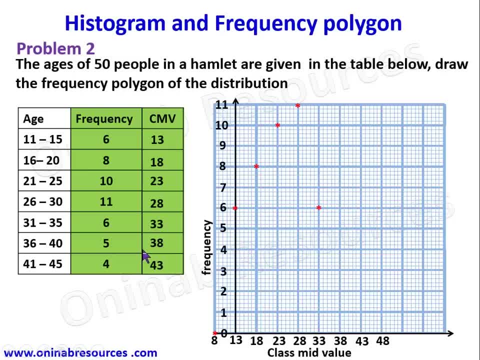 To get the midpoint of 0 and 1, we assume there is a number 0 before 1.. We are going to find the midpoint of 0 and 1.. To get the midpoint of 0 and 1, we assume there is a number 0 before 1.. We are going to find the midpoint of 0 and 1.. 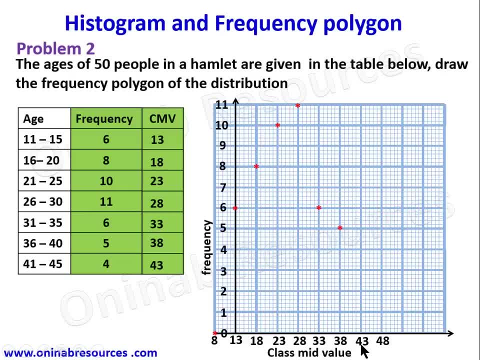 To get the midpoint of 0 and 1, we assume there is a number 0 before 1.. We are going to find the midpoint of 0 and 1.. To get the midpoint of 0 and 1, we assume there is a number 0 before 1.. We are going to find the midpoint of 0 and 1.. 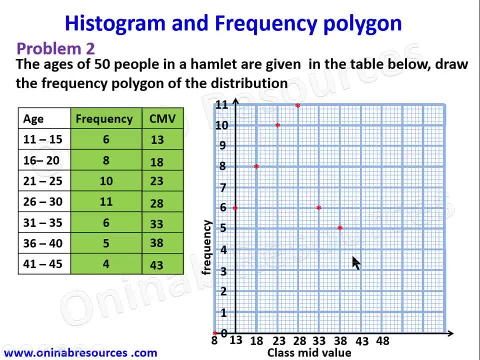 To get the midpoint of 0 and 1, we assume there is a number 0 before 1.. We are going to find the midpoint of 0 and 1.. To get the midpoint of 0 and 1, we assume there is a number 0 before 1.. We are going to find the midpoint of 0 and 1.. 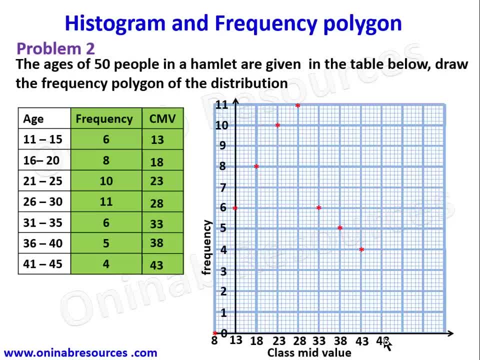 To get the midpoint of 0 and 1, we assume there is a number 0 before 1.. We are going to find the midpoint of 0 and 1.. To get the midpoint of 0 and 1, we assume there is a number 0 before 1.. We are going to find the midpoint of 0 and 1.. 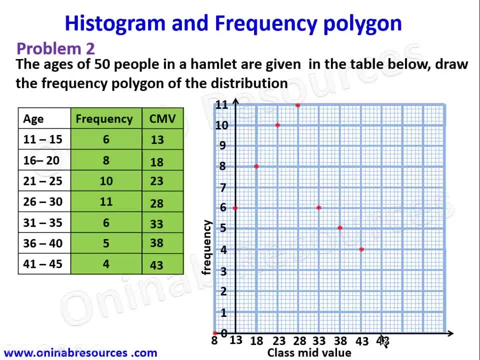 To get the midpoint of 0 and 1, we assume there is a number 0 before 1.. We are going to find the midpoint of 0 and 1.. To get the midpoint of 0 and 1, we assume there is a number 0 before 1.. We are going to find the midpoint of 0 and 1.. 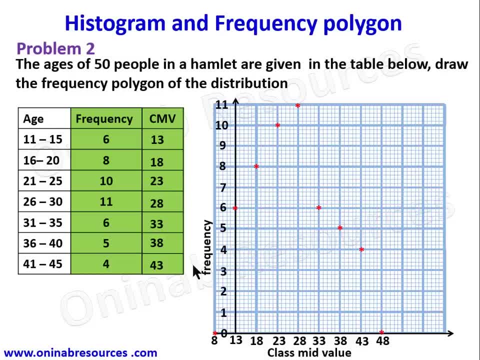 To get the midpoint of 0 and 1, we assume there is a number 0 before 1.. We are going to find the midpoint of 0 and 1.. To get the midpoint of 0 and 1, we assume there is a number 0 before 1.. We are going to find the midpoint of 0 and 1.. 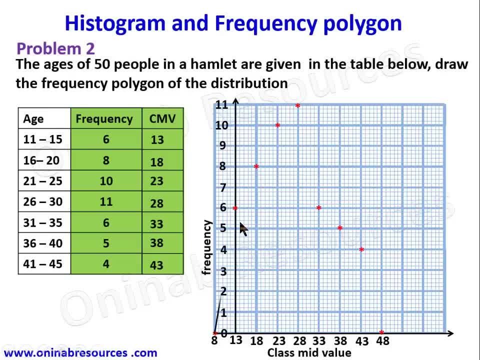 To get the midpoint of 0 and 1, we assume there is a number 0 before 1.. We are going to find the midpoint of 0 and 1.. To get the midpoint of 0 and 1, we assume there is a number 0 before 1.. We are going to find the midpoint of 0 and 1.. 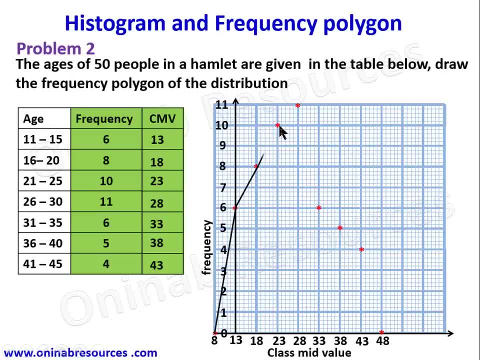 To get the midpoint of 0 and 1, we assume there is a number 0 before 1.. We are going to find the midpoint of 0 and 1.. To get the midpoint of 0 and 1, we assume there is a number 0 before 1.. We are going to find the midpoint of 0 and 1.. 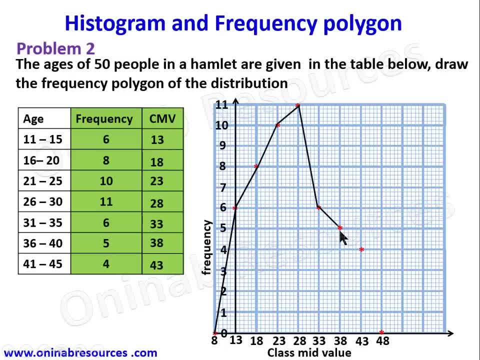 To get the midpoint of 0 and 1, we assume there is a number 0 before 1.. We are going to find the midpoint of 0 and 1.. To get the midpoint of 0 and 1, we assume there is a number 0 before 1.. We are going to find the midpoint of 0 and 1.. 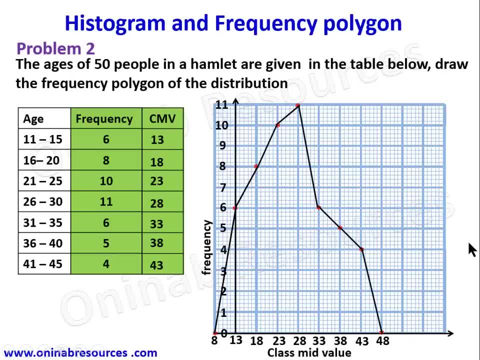 To get the midpoint of 0 and 1, we assume there is a number 0 before 1.. We are going to find the midpoint of 0 and 1.. To get the midpoint of 0 and 1, we assume there is a number 0 before 1.. We are going to find the midpoint of 0 and 1.. 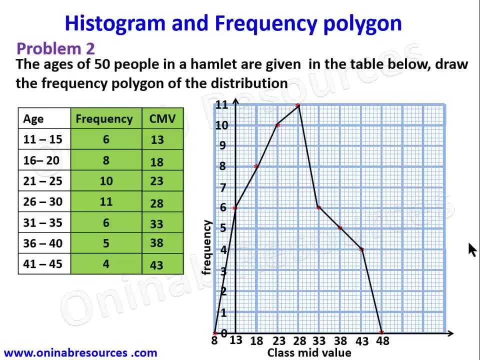 To get the midpoint of 0 and 1, we assume there is a number 0 before 1.. We are going to find the midpoint of 0 and 1.. To get the midpoint of 0 and 1, we assume there is a number 0 before 1.. We are going to find the midpoint of 0 and 1.. 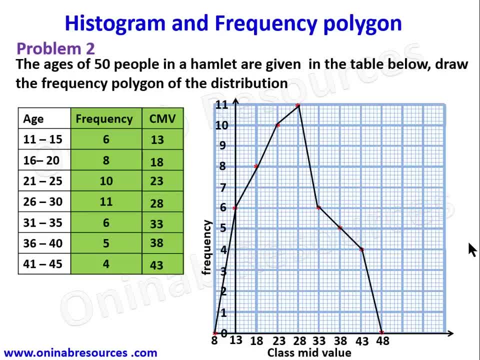 To get the midpoint of 0 and 1, we assume there is a number 0 before 1.. We are going to find the midpoint of 0 and 1.. To get the midpoint of 0 and 1, we assume there is a number 0 before 1.. We are going to find the midpoint of 0 and 1.. 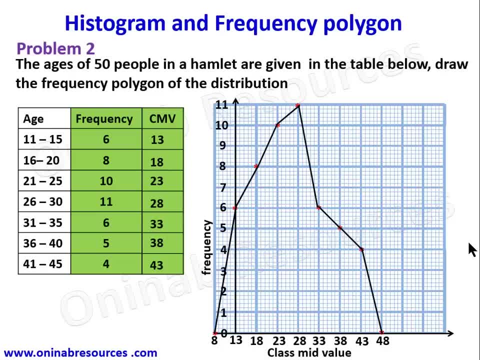 To get the midpoint of 0 and 1, we assume there is a number 0 before 1.. We are going to find the midpoint of 0 and 1.. To get the midpoint of 0 and 1, we assume there is a number 0 before 1.. We are going to find the midpoint of 0 and 1.. 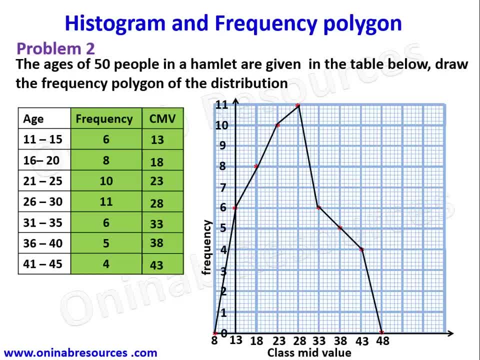 To get the midpoint of 0 and 1, we assume there is a number 0 before 1.. We are going to find the midpoint of 0 and 1.. To get the midpoint of 0 and 1, we assume there is a number 0 before 1.. We are going to find the midpoint of 0 and 1.. 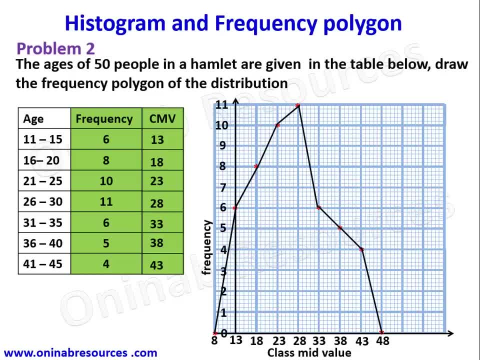 To get the midpoint of 0 and 1, we assume there is a number 0 before 1.. We are going to find the midpoint of 0 and 1.. To get the midpoint of 0 and 1, we assume there is a number 0 before 1.. We are going to find the midpoint of 0 and 1.. 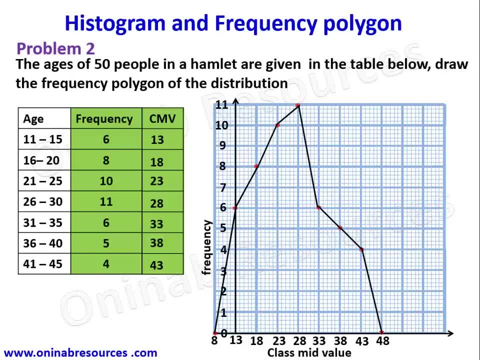 To get the midpoint of 0 and 1, we assume there is a number 0 before 1.. We are going to find the midpoint of 0 and 1.. To get the midpoint of 0 and 1, we assume there is a number 0 before 1.. We are going to find the midpoint of 0 and 1..